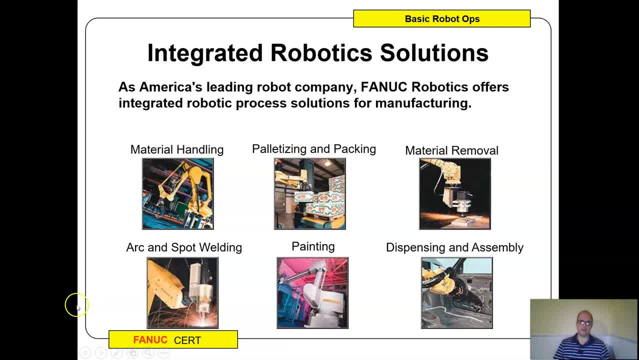 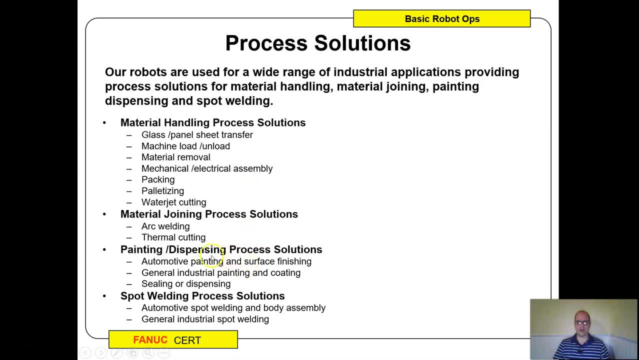 Robots are taking jobs, they're creating jobs and that's why you're in this classroom, so you can learn and be on the cutting edge of the future. You know- again here's a list of stuff we just talked about. You know, I've seen them in the RV industry. I've seen them. you know automotive industry. you know they're integrated with cameras. they're in the pharmaceutical industry, you name it, and there's a need for it somewhere. 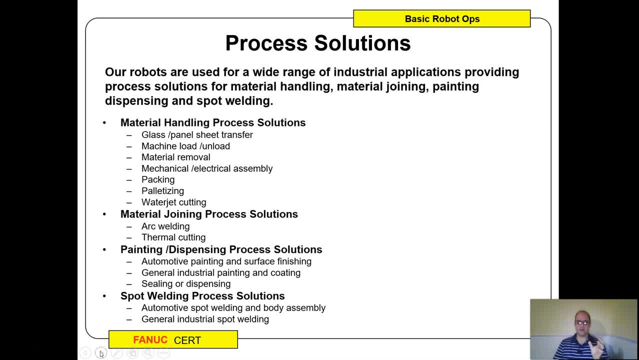 So don't just think of it as that. what we show you in this course, what you see, Know that there are applications that haven't been created yet, that we can use these for. Material handling is the biggest one. you know. palletizing, you know. 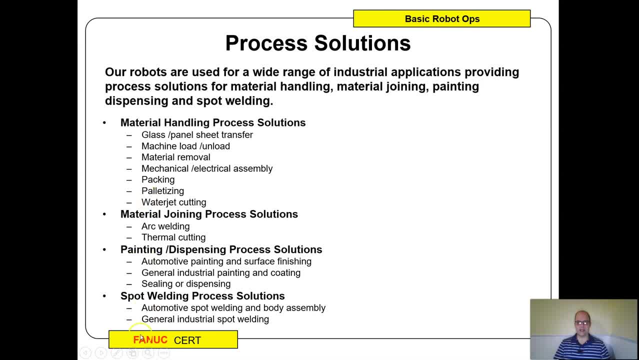 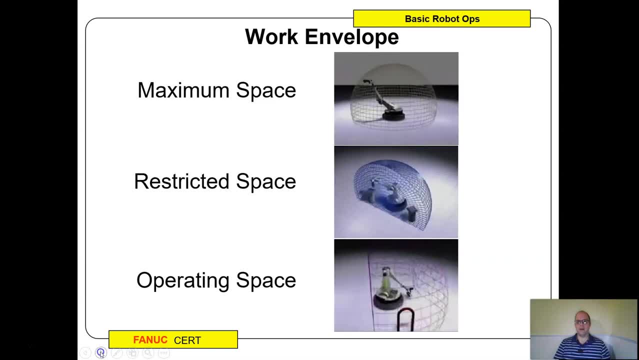 Removal of material, that's the biggest one. but all these, welding is another big one. but all these are applications that we can utilize this for Depending on, but some, some. let's talk about some, some terminology. The maximum space of the robot is, if I extend things out to the maximum, like the part of this reach that can go. 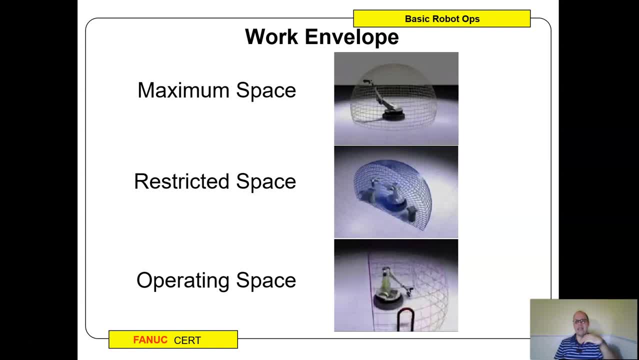 Will it ever go that way? Probably not, but you have to take it into account. You know so. if I, you know so if I lay down completely, You know I can extend more than if I'm just in this area right here. 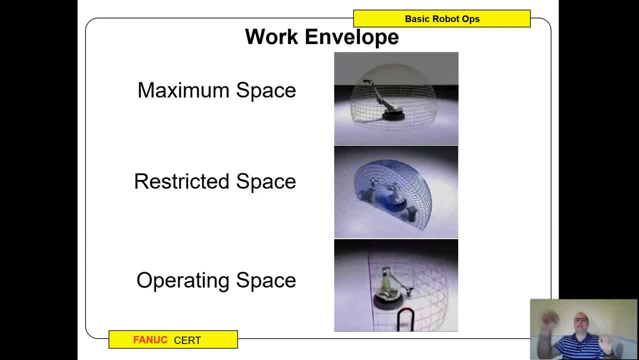 And think of it that that maximum space is, if I totally lay out for something, the furthest it could reach and hit may not be operational, but it's the furthest I could hit and reach. The restricted space is where we try to keep a robot too. 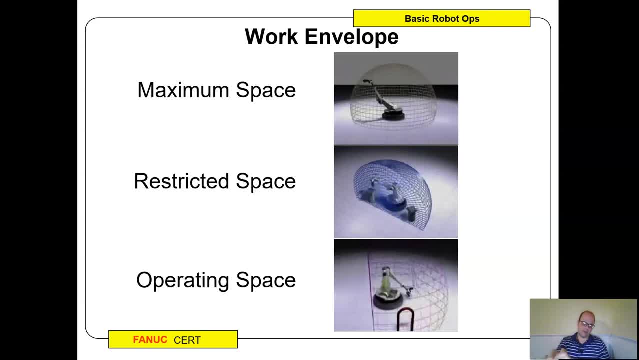 So that may be what's what's been guarded, or it's not past its maximum space, but it's a space of where all the work is, It can be done in reality as it moves, And now the opportunity. So the operating space is, in general, the space at work. 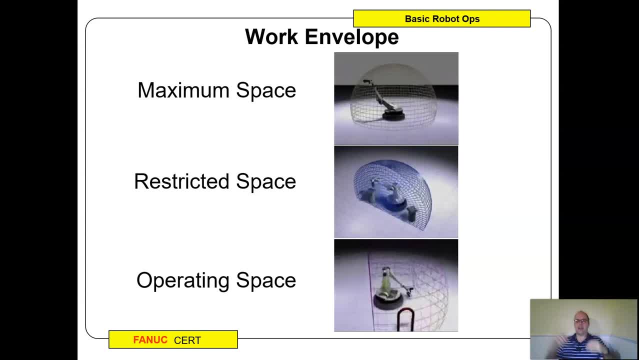 So think of it as slowly clamping down on stuff So like. so if I lay out again, that's maximum space, Restricted space is like this little corner right here. My operating space is right here on the keyboard, If that makes sense. 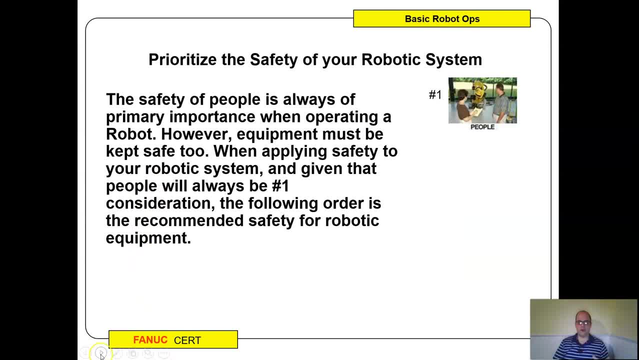 Um, but the number one rule for robot, for for robots- is the safety of the operator comes first. robots can be replaced or expensive parts can be remade, but the you cannot be. Uh, we don't live in a world yet where we can reach where you, we can replicate you, so you are the number one concern. so everything is takes that into mind and we want to make sure that you are the next, the person that is safe. 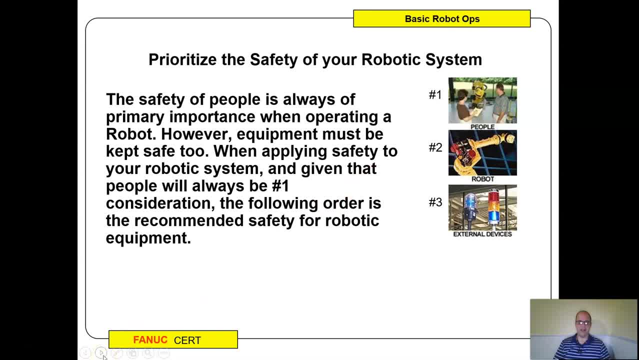 The robot is next, obviously, because there's a big piece of equipment: external devices like stack lights, you know fixtures um, the controller, you know safety, that's next, um. but the tooling is last because that's the thing that attaches to the end of the, the uh robot. 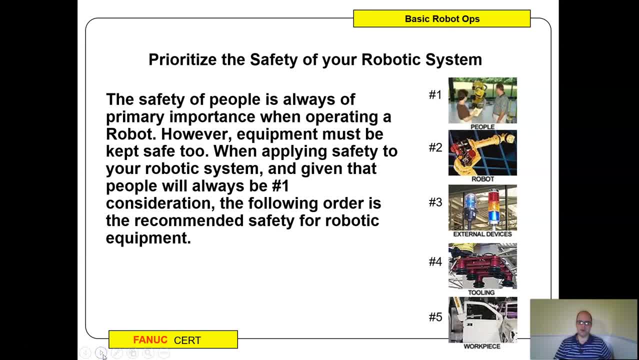 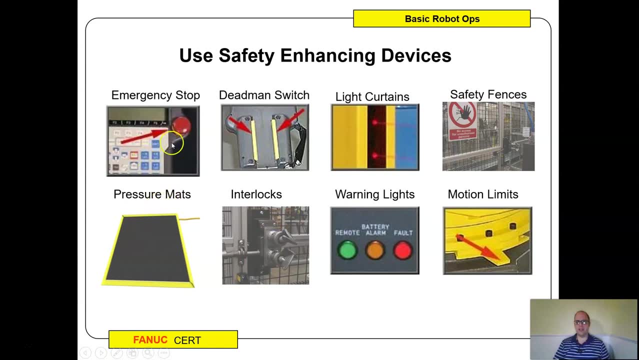 And then the work piece, because the work piece is what we're. we're fixing or moving. We can replace that a lot easier, but that's the. this is the priority of safe priority of a robotic system. Um, these are all things that you will see around this, the. you know everything. this is called the teach pendant. 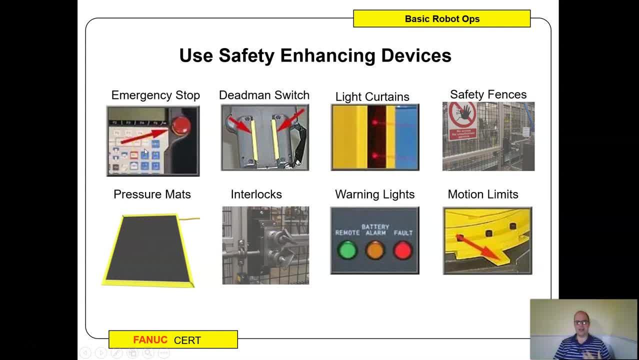 We'll talk about that more a bit. There's an e-stop on it that allows you to stop everything If you think the robot is coming down on you. the dead man switch right here. that is going to be the thing that You're going to struggle with when we start jogging the robot, because there's three positions. um, all the way out means that Hey, robotic can be by you. 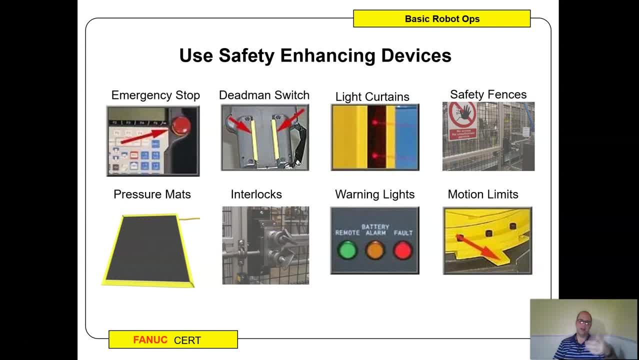 Don't move. I'm not touching it, you know. so don't move, because I could be by you If I push it all the way in. um, it's saying that my arm or my muscles are cramping up because I'm being crushed or electrocuted. 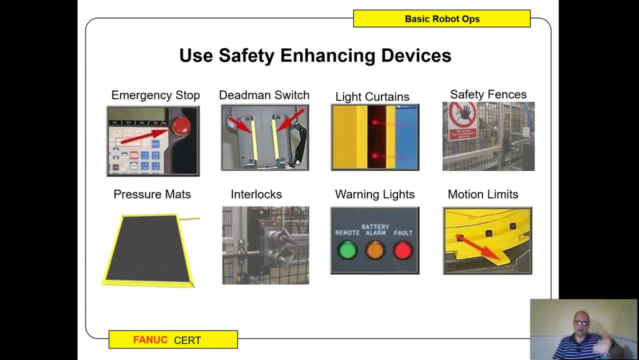 So, robot, stop doing what you're doing. The sweet spot is in the middle And literally, if you just let the weight of the teach pendant just kind of kind of rest on your hand, it will Click into that middle position and that will allow you to move things. 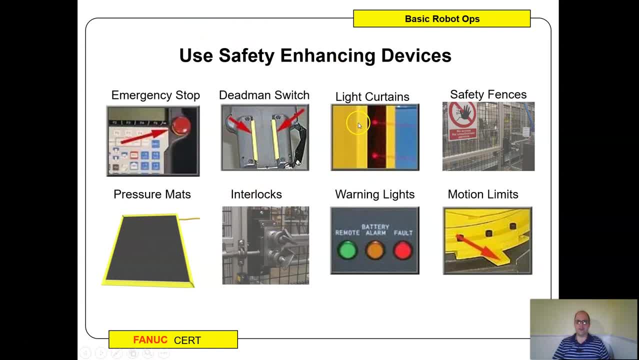 We'll talk about it more in class. Um a light curtains are often used because if you enter into the light curtain it could stop things. safety fences, pressure mats making sure that you're on there. Interlocks- meaning that you know both keys have to be turned. warning lights, motion limits- like physical, like screws that keep the robot from moving past things. 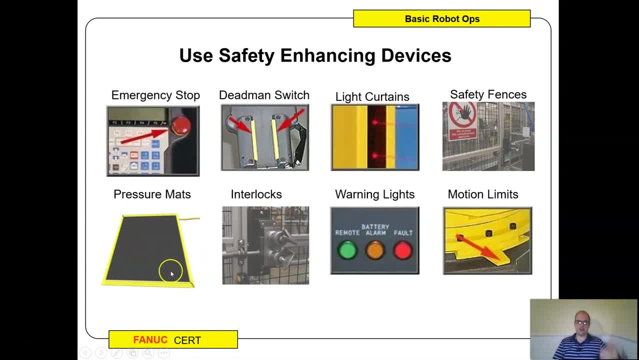 All of these are meant to keep the robot safe and making sure that you're not in the way of the robot when it moves. Now there are a lot of robots are being It's now that called collaborative robots- that have extra pressure sensors and safety sensors and speed sensors in there so that if you run into it it will stop. 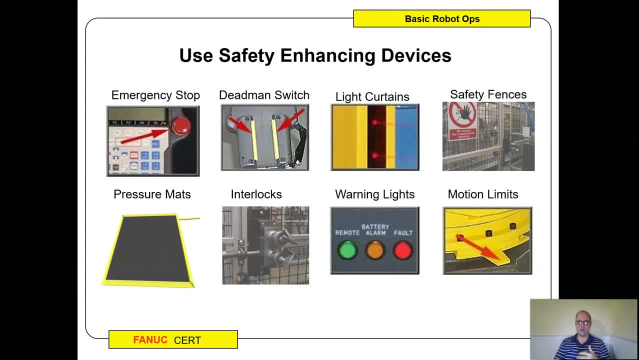 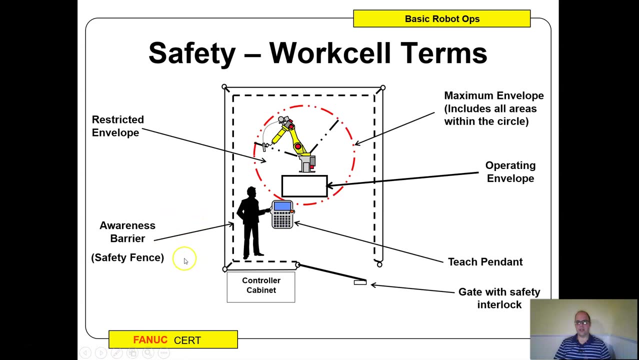 And I might share a video of that- when I got a play with one at Vanix headquarters And, by the way, it's pronounced panic, not for Nick, panic. Um. so there you go And I'll advance through it, but some here's some other things to think as you go in. if you go into 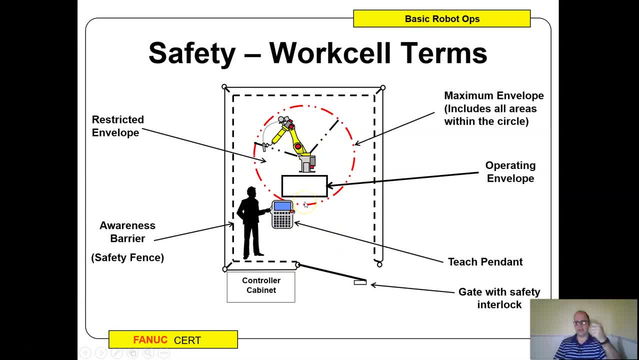 The area where the robot is. you always take the teach pendant or some type of e stop device. Ideally it's always a teach pendant. Usually there's a safety gate with interlocks. There's usually a barrier fence with it And you know, that's the. that's there's guidelines with us, with the, the robotic Institute of America. 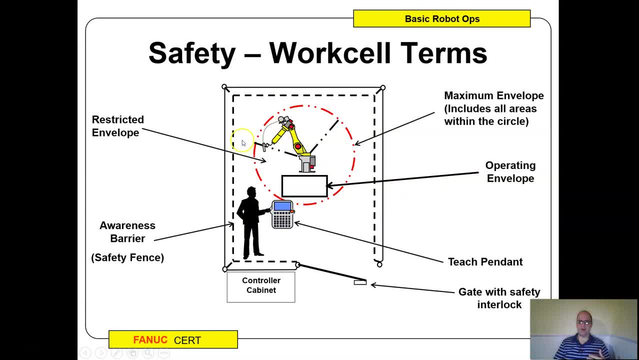 They're all on their website. You can check them out. The maximum envelope, though, is all the areas that it's going to move around to. there's the operating envelope is where we do the work, Is it? Most robots are not going to go around. 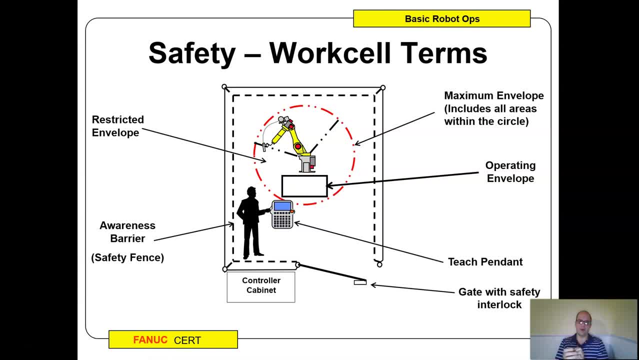 All the way. Usually we focus our attention to 1 area because we don't want. we want cycle times below, So we're not making a move all over the place. Um, the teach pendant, and then there's the controller cabinet. The controller is the brain of the robot. 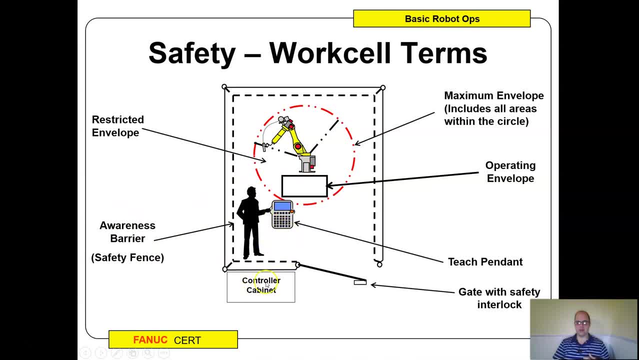 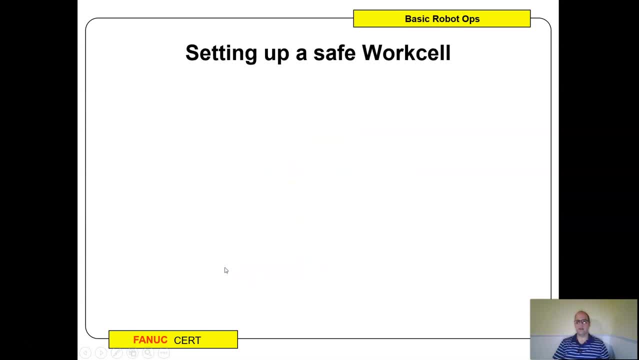 Usually the teach pendant is attached to the controller cabinet and then there's a cable that attaches to the robot that says it sends everything. Okay, so setting up a safe work cell. these are things. Oops, let me go back. These are things that keep minds. 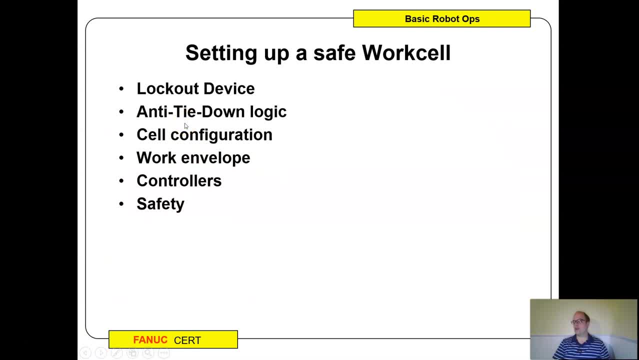 We just talk about and big thing is anti tie down logic. You know, all of us have been in a situation- maybe on the, in the farm or something like that- where you need an extra set of hands to work on something like maybe and, and and we we do something unsafe to, to keep something from to do things. 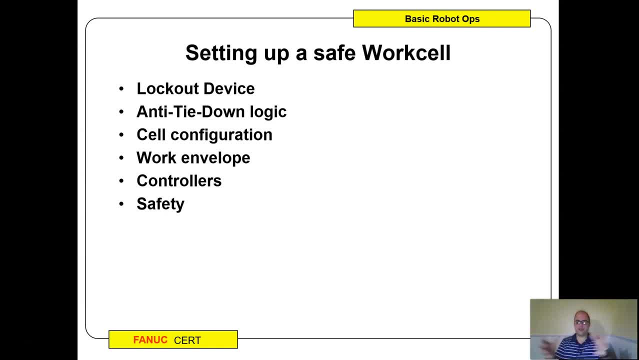 That's what tie down is. So a lot of times there will be, like you know, say, for example, the pressure sensor. you know you may try to do that Indiana Jones thing and put some something of the same weight on there. 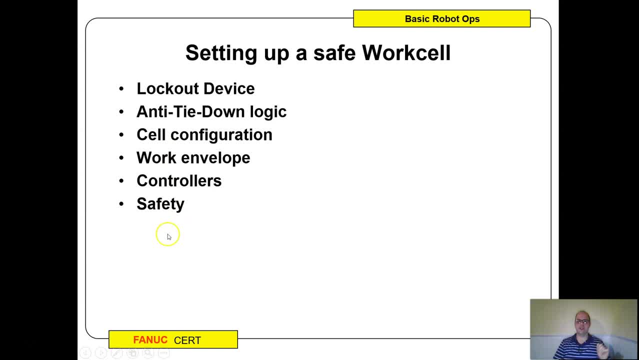 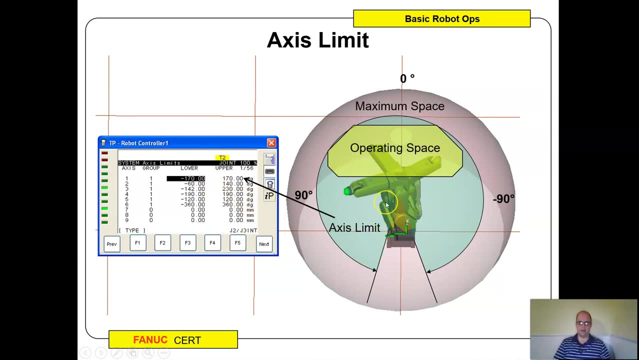 So you can actually work on the robot to bypass safety- Always a bad idea, So we look for ways that multiple safety mechanisms to keep that from happening- that you cannot bypass them all. Okay, So access limits- this is one of the things you're going to look up. but we can program how far this robot can move. 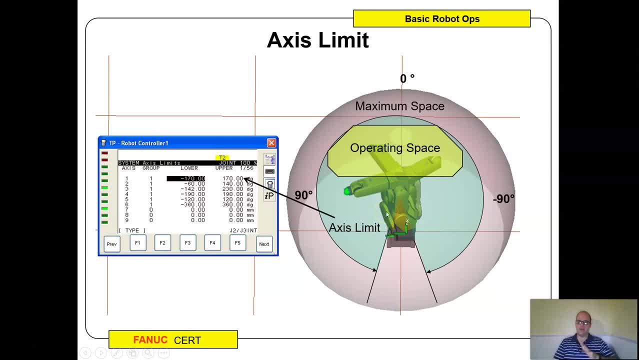 Usually, you know, we'll talk about the joints. Joints are set up in like a degrees, a degree situation. So again, 360 degrees is a circle, but if I can limit, You know it to be, and we won't do a full 360 degrees, because which is zero, which is one's, usually it's 180 to one side, a hundred and negative 180, and that equals 360.. 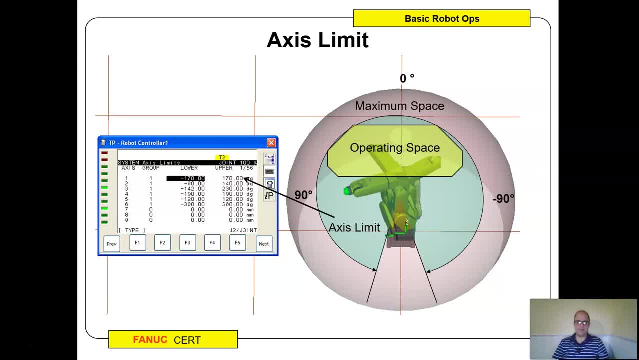 So we have a positive 90 or positive, negative 90, but this is saying that we're going to restrict access- one which we'll talk about in a second- to only 170 to, you know, and 170 negative. So access to would only be 60.. 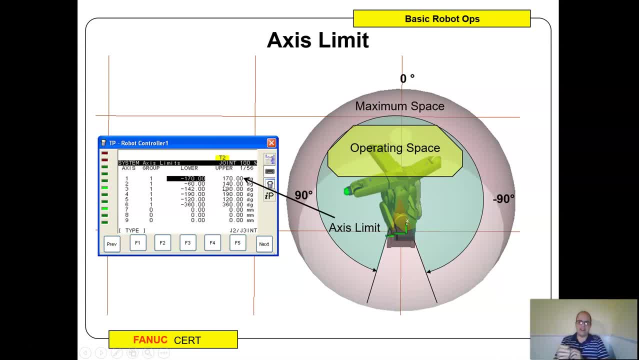 These are all set up from the manufacturer. You can zone it in more, but then there can be some issues later on, So do this sparingly. We will do this in the class so you can see it in action, And usually you have to cycle power on the robot for those that come into place. 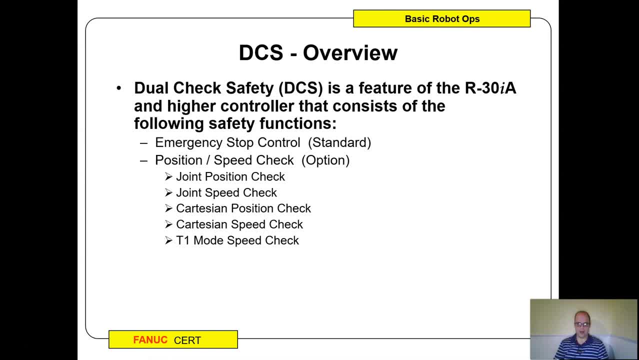 One thing that panic uses something called dual check safety on their robots. It is what it does is it checks the speed of the robot and the position of the robot at points and creates an extra layer of safety. It's a. It can be fun, it can be challenging, but it's also there for your safety. so you can see it has position checks and speed checks and Cartesian check and speed checks and other things so that with the robots moving, it won't let it happen in an unsafe way. 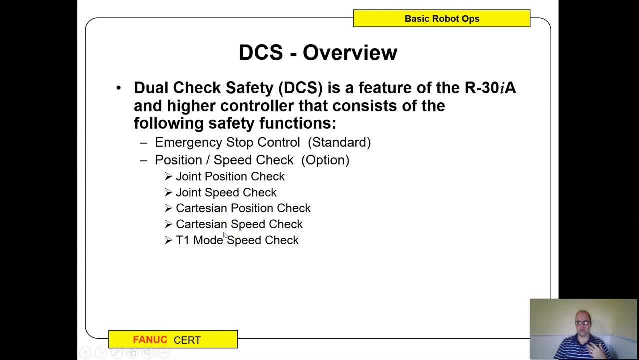 You know what you'll find is these newer robots know exactly where all of its joints are in space and it knows that parts of it. So say that that we, we set up a DCS zone around here And if I'm moving the robot and it gets there, 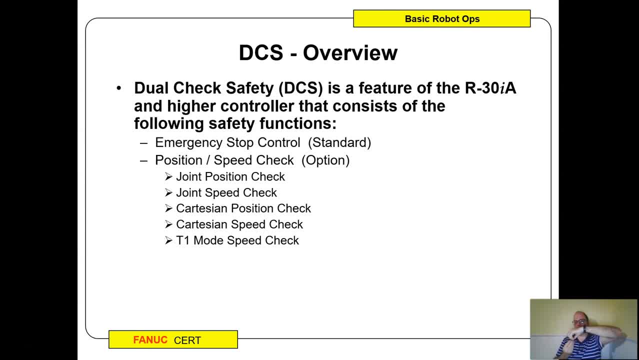 A part of it. A person could be here even though the work is being done on the end of arm tooling here. It knows that the robot is leaving the zone, So it stops the robot from moving anymore. That's one of the cool things about dual check safety. or if it's moving super fast and it may exit that zone because it's got too much area to go, Not enough Stop, It'll stop in time before it gets out of that. So do those calculations for you. 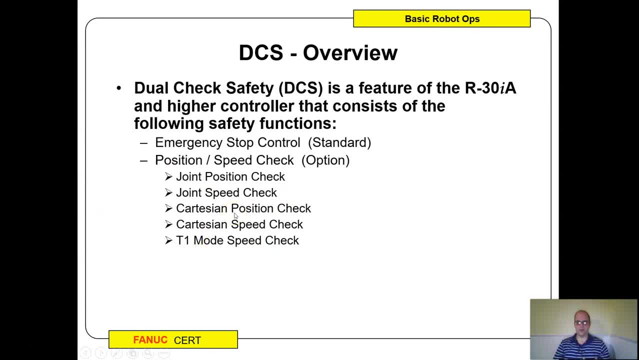 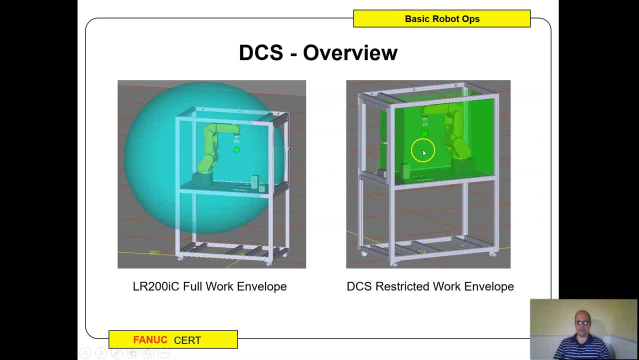 You'll find DCS errors. that happen quite a bit because they're on our robots. You know you can see the full And this is like A certain cart. you can see the full work envelope. Here's what the DCS restricted is, So it keeps it from going out the side and everything else. So it's just another way Cause like if that robot turns it could hit the wall even though the work piece could still be doing work. 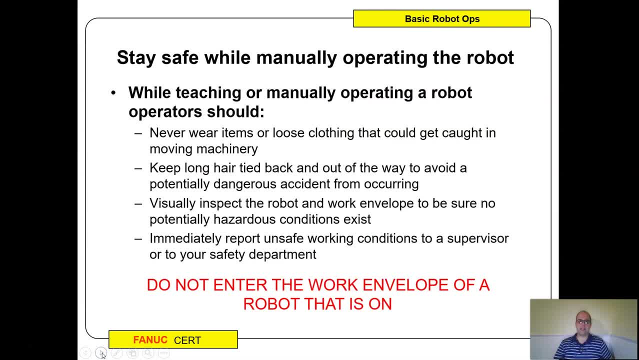 You'll find that out the hard way. Some things to keep in mind. you know, never wear loose item or jewelry. you know long hair visually inspect, And the biggest thing, though, is: do not enter the work envelope of a robot that is on. 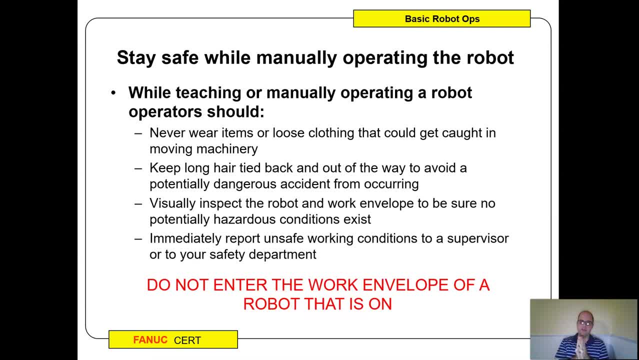 We are an educational environment So we do have some big robots, but most of our robots are small. You can get lulled into a sense of safety And forget that this is a robot that can still hurt you. So in class never boot the robot up and auto without me for checking it. 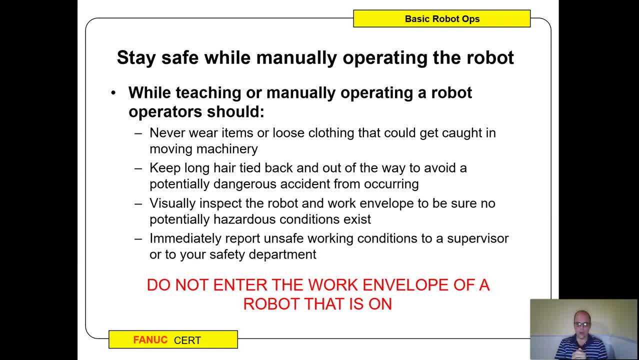 And always, always, always, always, always, always, Have the safety gates closed. If you're moving the robot in automatic, when you're in manual mode or teaching mode, We might need to get in there and look at something, or when we start doing frames, you might need to get in there look. that's understandable, but you need to be careful and never, ever, ever. 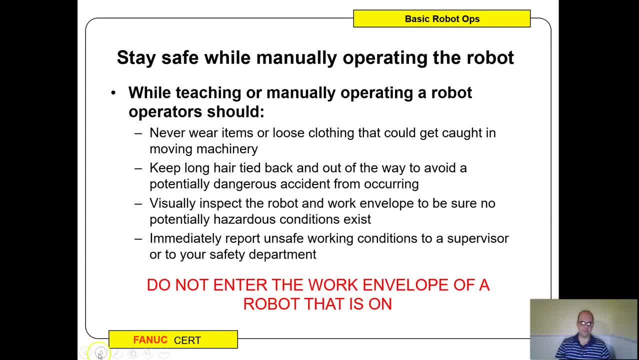 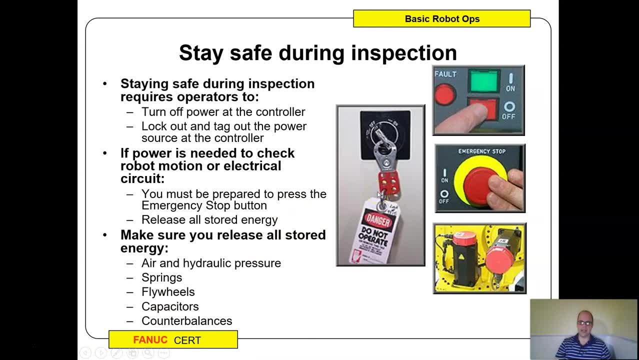 Be in a robot cell longer than you need to be. Certain things to do. You can lock out, tag out. It's not intuitive on the fan of controller, but you can lock out, tag out If you need to work on a robot. good practice. 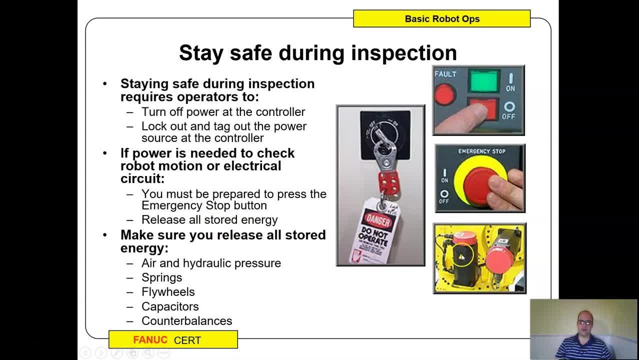 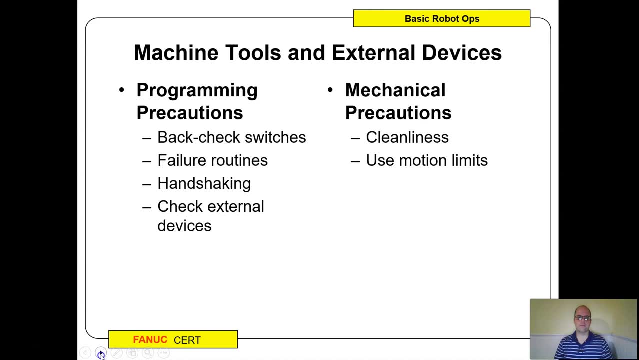 But in some cases you know, you know so, like if you're replacing a servo motor, you need to lock out, tag out. no electricity gets through the system. make sure any flywheels or capacitors or counterbalances or springs are loosened as well. um sorry, um program precautions when you're programming. 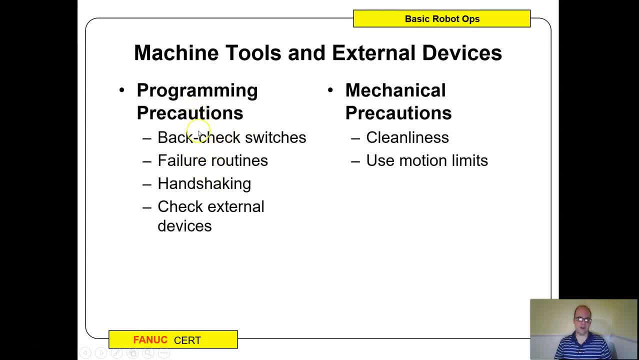 make sure that there's um, you know there's some program precautions you can take place and there's also and you want to make sure things are clean and motion limits protect things. so you know when you're programming, make sure there's handshaking going on between the robots, that there's external 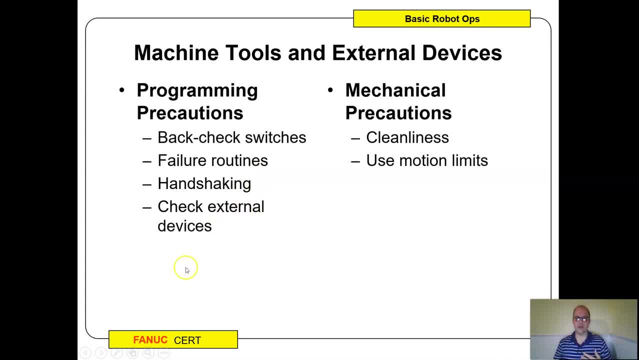 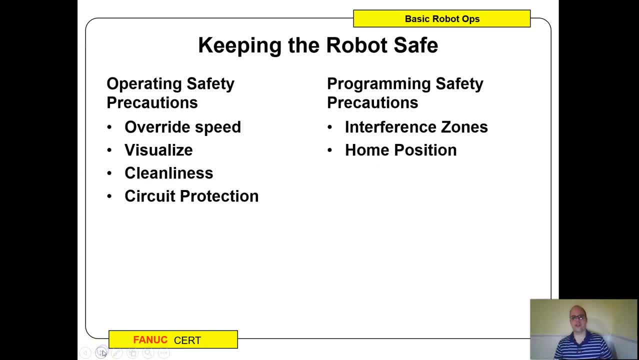 devices in to keep things safe, so that you're doing, you're making the setup so you're not going to hurt things, you or the parts when you're keeping the robot, to keep the robot safe. you know, be careful. the override speed which we'll talk to visualize where you're going. make sure things are. 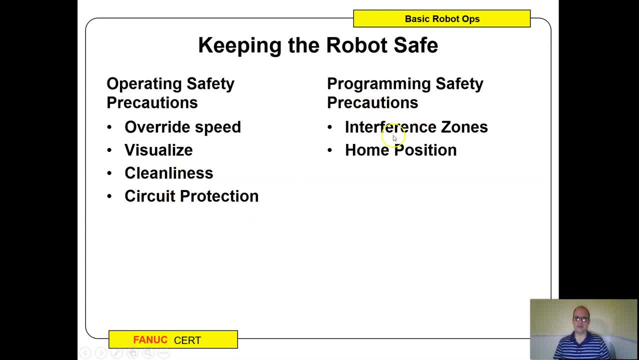 clean, make sure circuit protections are in place and when you're programming there's things called home position interference zones that we're not going to get into this class, but these are things you can do to make sure that the robot is safe. so if one robot enters the interference zone, 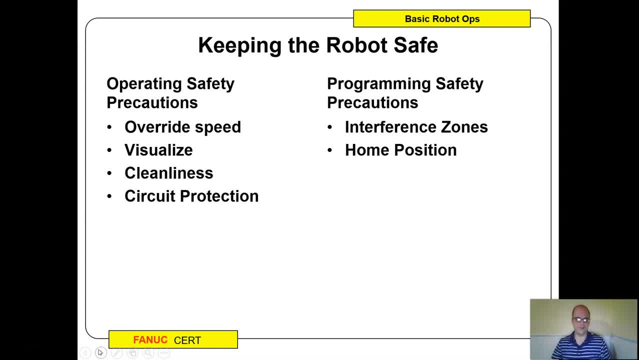 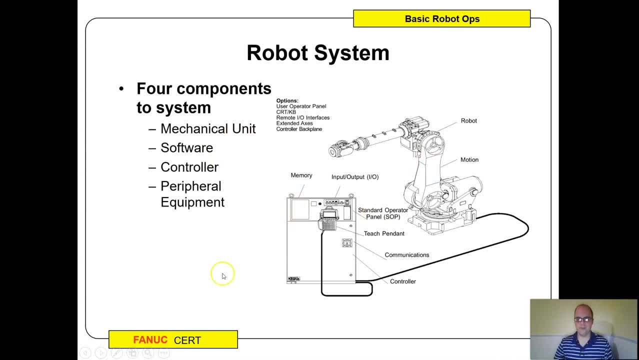 it keeps another robot from entering or other things from taking place. i o signals and things like that. so here's the general robot system. we got the mechanical unit. i think it highlights: oh nope, wrong mechanical unit. there's a software that runs off the controller. um, this is the controller and there's peripheral equipment. 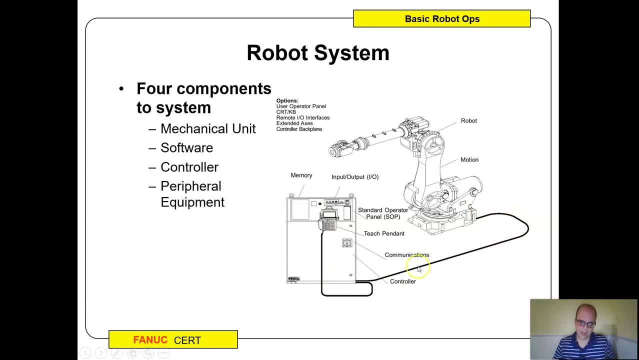 the teach pendant is peripheral equipment and, as you see before, here's a cable going to the controller and a cable going to the teach pendant. all right, the teach pendant is how we will program the robot. it's basically like a big, giant video game controller. you will see that, um, man and when. 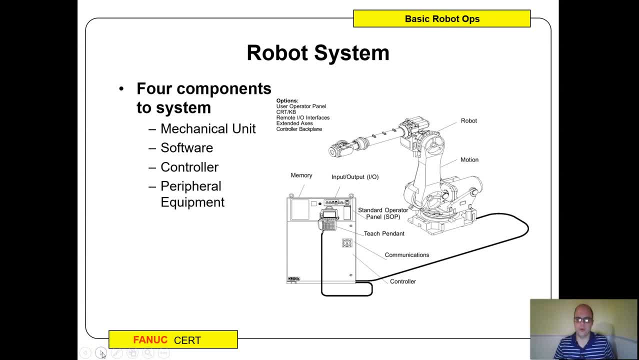 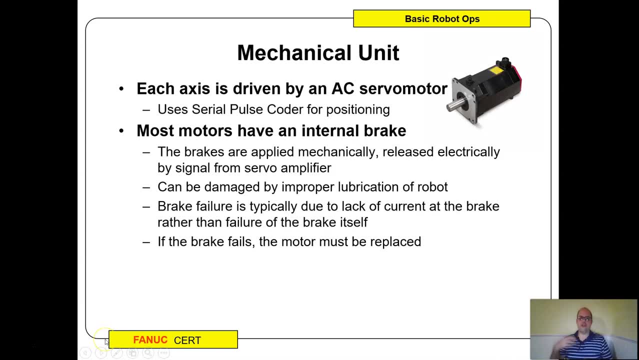 we program is jog the robot to a position and hit some buttons to store where it is and how it gets there. we'll talk about that in a few weeks. um, when it comes to a mechanical unit, howard knows its locations, it utilizes servo motors, ac servo motors. that that basically has a serial pulse counter. that. 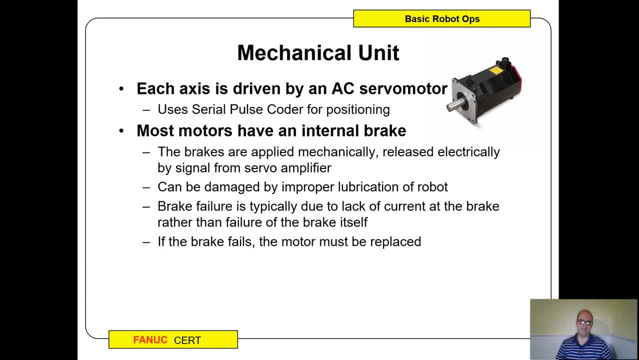 exactly where it is. so when you first turn on that robot you know it knows where it is because of the, because of how many counts of the pulse that has been set it. there are absolute numbers- that when it first is set up that it knows where things are. but if you ever change it out or do things it's. 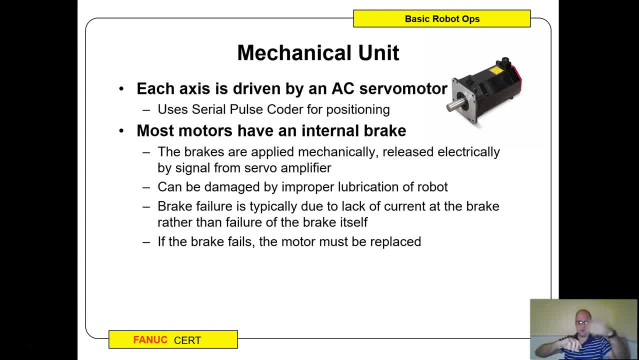 different, but but it will know by as you rotate. that's how it knows the degrees, how many times it pulse around, so it knows how far the robot is. that's all set up on the back end. um, that thing is. it has an electric motor, but it also has a mechanic on a brake. so every time that you apply, 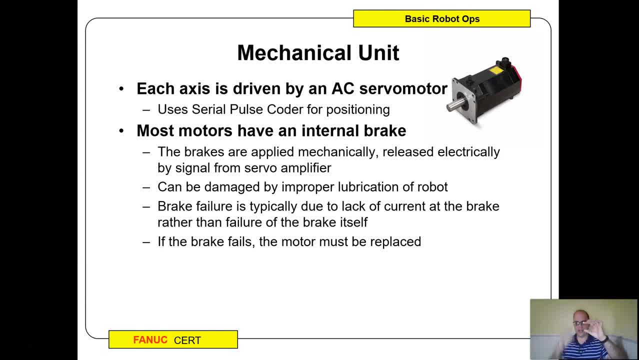 turn on. you know, turn on the servos, the brake, a brake is dropped and and the servos are applied, the energy is, uh, supplied. so it is a mechanical system, but you got to understand that there's a brake and then a motor goes. so if any one of those things don't work, like if you don't have power and 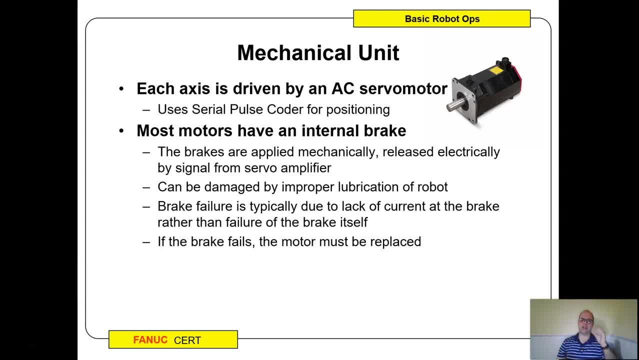 the brake disengages, your robot's going to drift. if you're, if your brake doesn't disengage and you're, you're going to have like. you know that it's like you driving without your emergency brake on in your car, it's going to cause some issues, um. so you know you need to. 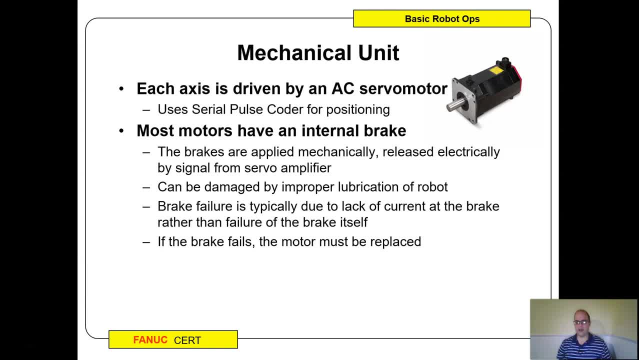 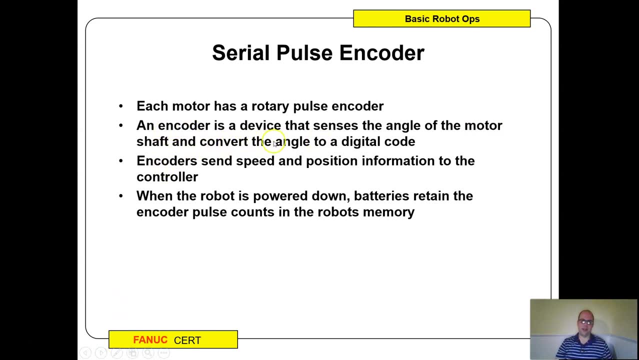 lubricate, uh, not the servo motor itself, but the, the joints that. those are all part of the pm of the robot. but this is a mechanical unit. that is you that is utilizing power to make your life easier. so, these serial pulse encoders- there's a rotary post encoder, you know, and the one thing, 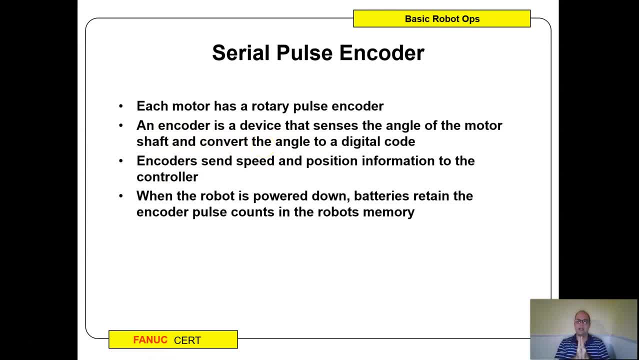 that i need to express to you right now that the robot is programmed to know where home is. there is no home unless you tell it. out of the box, there is an absolute zero setup where it kind of straight on and upright: um, that is a way for us to check to. 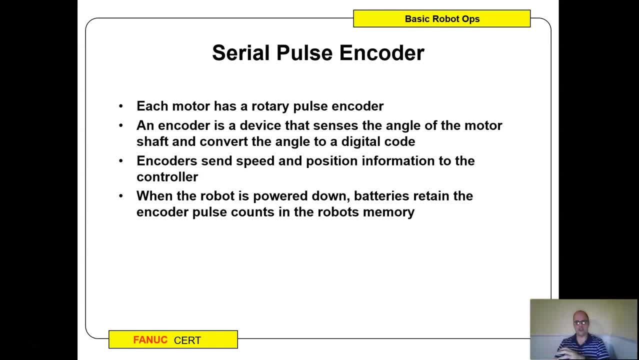 see if it physically knows where it is in relation to the software. it's a double check, it's a calibration point, but in some cases you know you could, you can go out industry in the robot's home- it's like this or something else- because it's hanging upside down. so while we do stuff in the 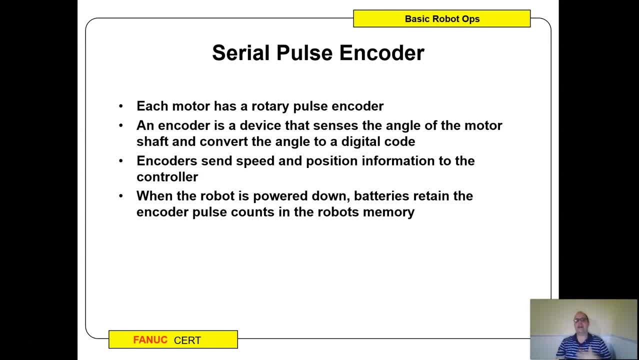 classroom where it looks like it's all zero and that's the normal set. that may not be it in the real world. physical markings can change, so, um, all those are set to do is is that, when the robot wakes up or where it knows that, we can have a double check to know it's there, because the robots have. 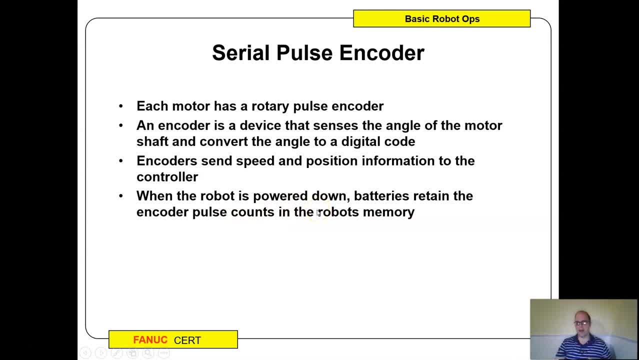 batteries. in reality we're going to keep the robot's home for a long time, so you know that's on at all times so it remembers where it is. but if power goes out and robots go asleep, there are in our robots there are four c cell batteries that are in the base of the robot. 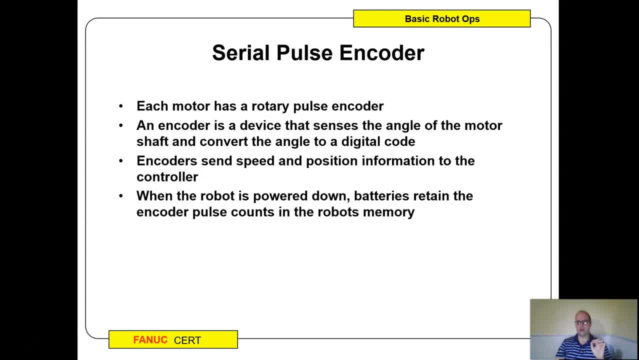 that when it powers down, it powers the encoder, so it remains where it is, so that when it wakes up it knows exactly where it is. otherwise it's to be like, you know, you ever fall asleep on your couch and your kid comes in and they wake you up. you're like: oh, where am i? you know, that's what the robot? 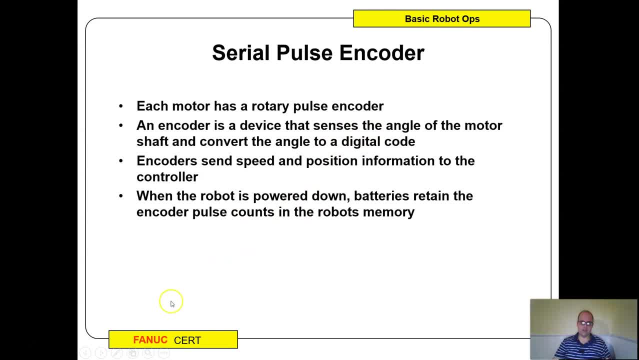 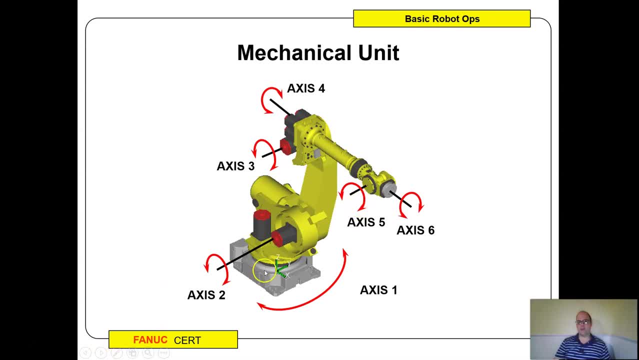 does. it causes an alarm if it doesn't know where it is, and so the pulse, and so there are batteries in the robot that restores all that information when it powers down. so let's talk about the robot itself. okay, this big axis around the bottom here, that's axis one that's, if, a twisting motion axis. 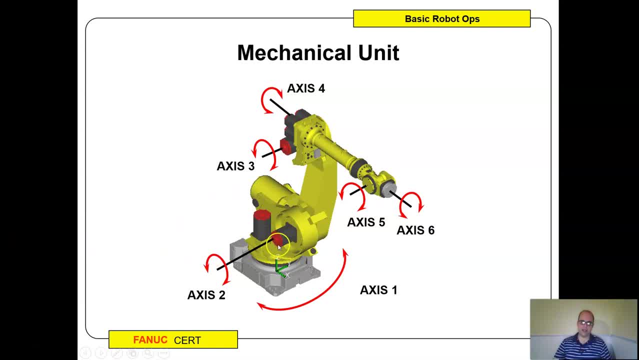 two is usually right here, usually right here, kind of a bending motion, um, uh actually, uh no, that would be axis three. no, x3 is up here. sorry, axis, that's the servo for one. axis two: sorry, it's more easier to see in real life. axis two is a bending motion. axis three is like a shoulder motion going. 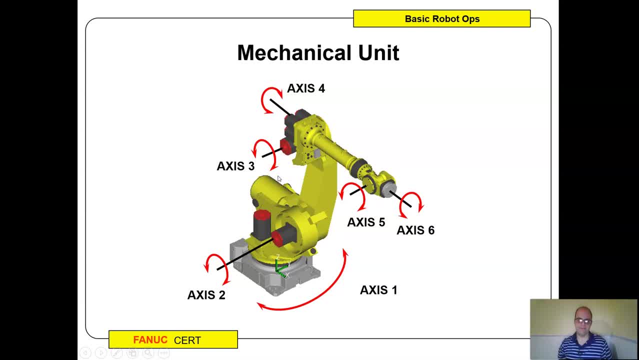 up and down. those are called your major accesses. all right, one, two or three, or major act, because they're their big motion types for the most part when the robot moves. those are the three accesses of moving. four is kind of it is kind of like a twisting motion or y'all. no, not necessarily. 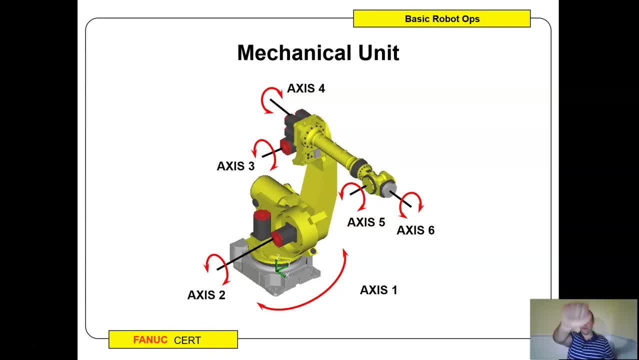 y'all yet. but this is a twisting motion. five is kind of a risk motion, like this, and six, six is like imagine if this rotates around and with those six degrees of freedom we can manipulate things to get wherever we need to be. um, and so, axis one, hip, um two. think of it as the 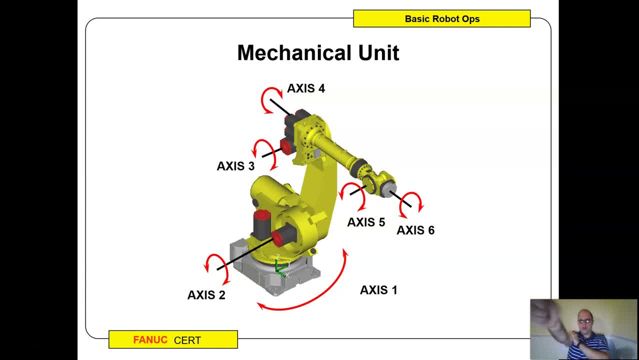 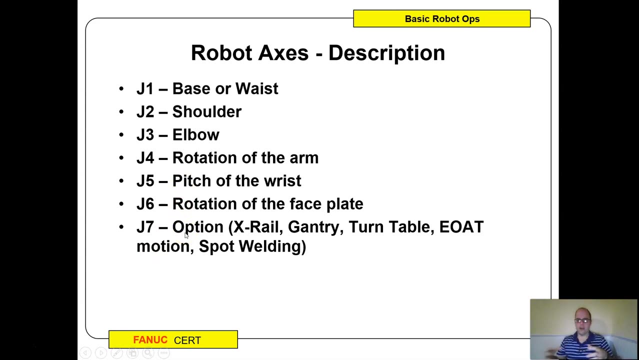 weight bending forward. uh, three shoulder, you know, a twist is four, wrist is five, and you'll hear i call it a wrist, and six is the face. play the robot, okay, as i just, and then sometimes you'll have uh the robot on like a gantry or you have a turntable. you can control that with joint seven. 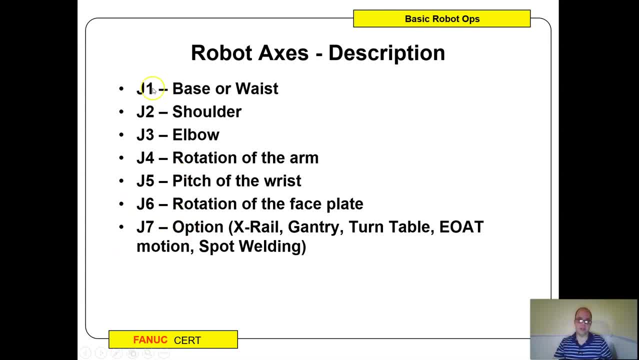 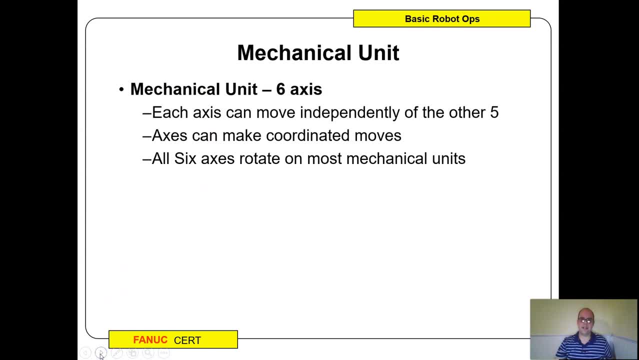 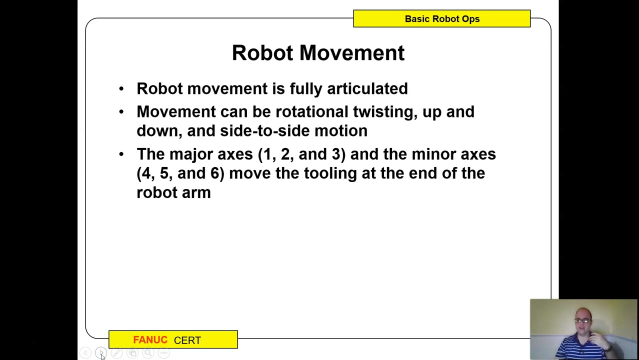 we're not dealing with that in this class. okay, so you know, here's everything in reality. um, and each axis can move independently, or what makes this fun is what the robot can do: calculations, so they can move together in coordinated motion. okay, um, you can have the rota, you can twist and go up down, side to side. you can articulate an. 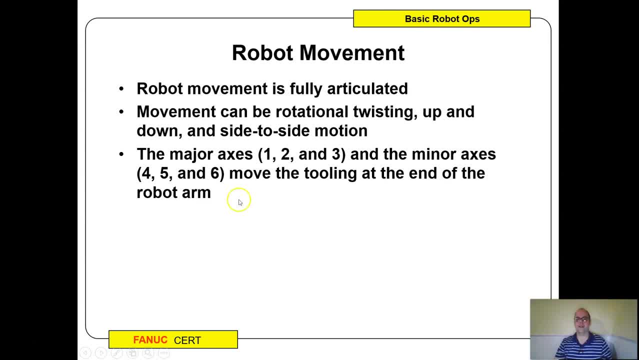 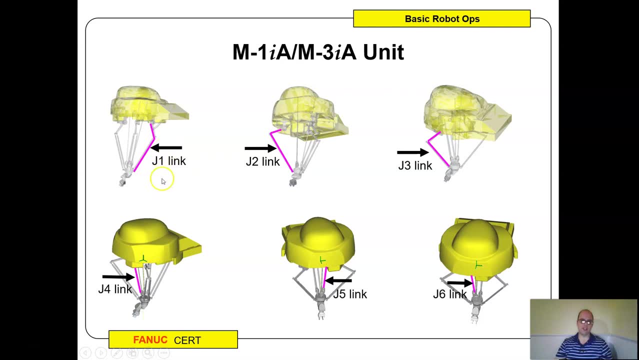 any way. um, but the big thing is, you know, there's the major accesses and the minor accesses. the major is the big motions, the minor is the small detail motions, that that have all the fun in the world if you're doing, uh, detail work. we do have one of these spider robots. we do not have a. there's. 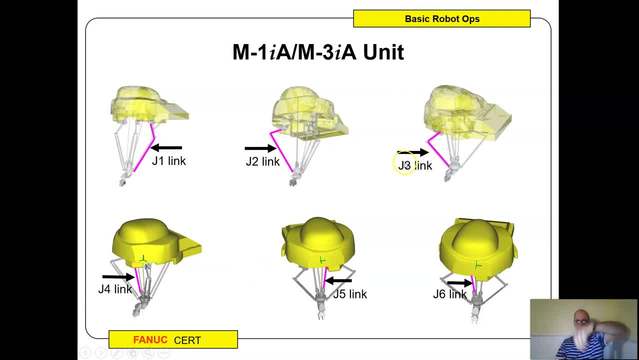 no joint four or joint five, but this is what that would do. this is a high speed pick and place the robot, um, and it just moves in three dimensions and twists. some of you will use that robot in class. uh, just simply because, um, the t-dependent is the same certain labs, i'll say we'll move on. 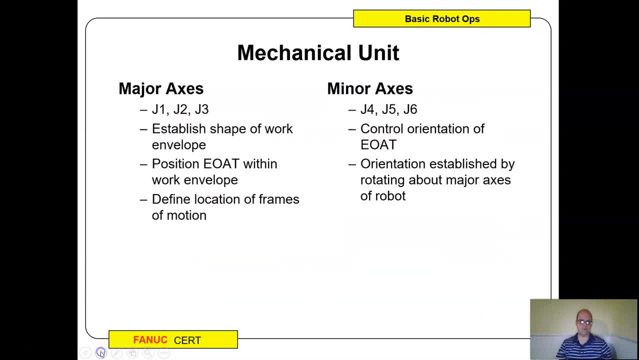 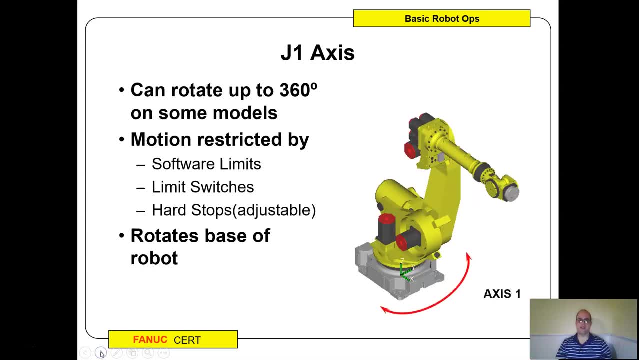 to the other robots, but that at least allows us some more flexibility in the classroom. okay, um, same thing here. a little bit of review. so, j1, you know you can go 100, 360 degrees, but probably won't. um, there are hard limits. is confined by this limit, switches on the on the bottom and hard stops that are adjustable. 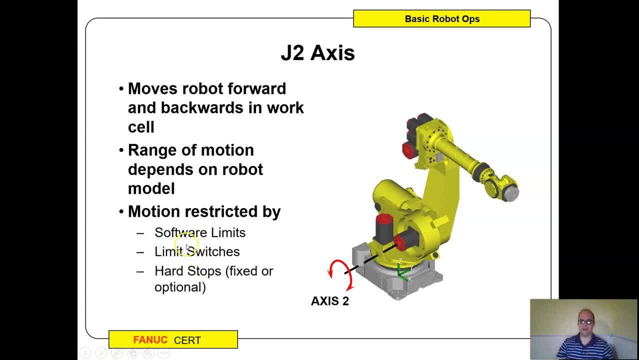 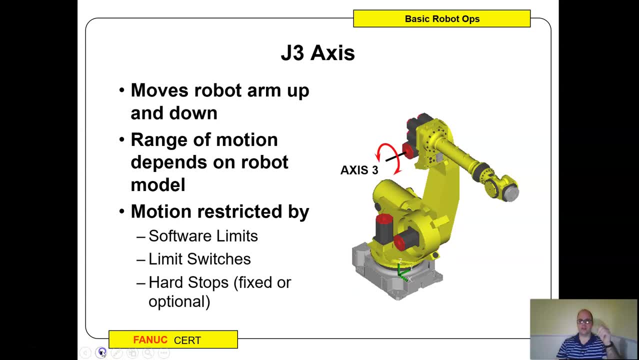 axis. two: um, again hard stops and limit switches, but that's how it's confined. same with three hard stops and limit switches, but moves it up and down. four: this is software limits. it could go around and around, but sometimes you don't want to go round and round, but this is only restricted by 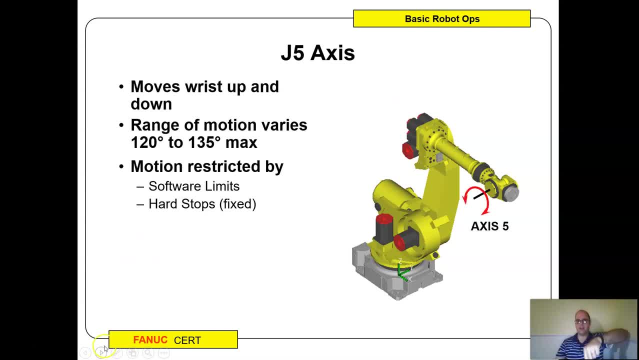 software motions. um five is hard because if- and it's gonna have a maximum range, like this, because you don't want it to bend up in itself, so there are hard, they're hard- stops and and and limits. um because you can't go in on yourself like 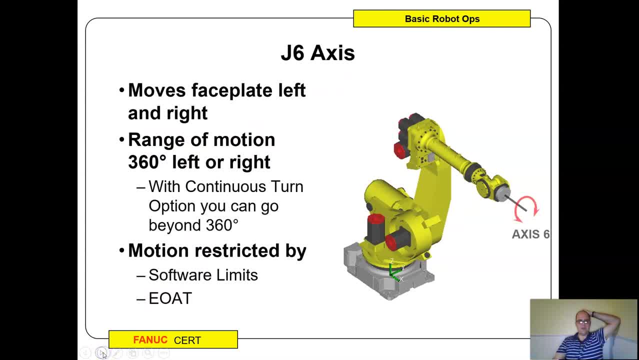 that and then the face plate will rotate continuously 360 degrees. but you can put limits in so you don't go too far and too much around. um, you know you can go beyond 360, but it's usually not recommended. sometimes when you're programming you might need to wind. 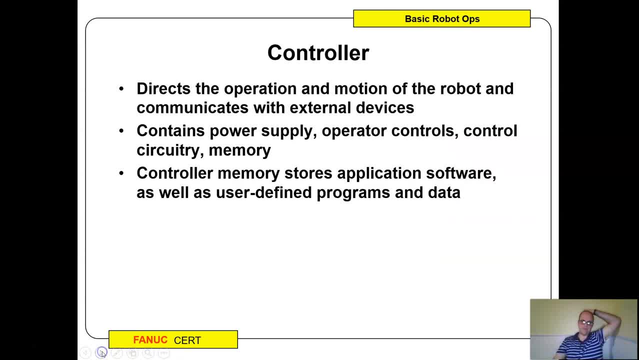 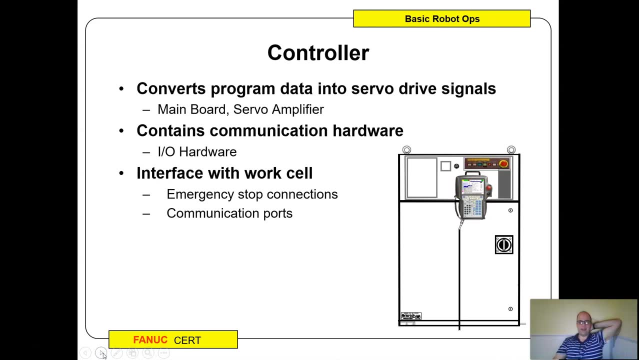 something up and then wind it out, or we'll hit these access limits. okay, the controller will directly communicate everything, and this also houses the power supply, the transformers, um memory, all that fun stuff. um, the io board goes through there. um, you know we're going to talk about. 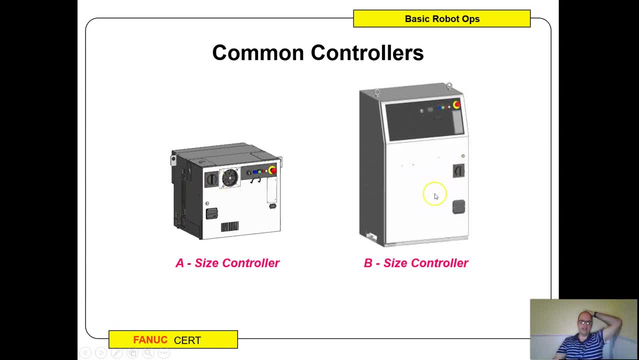 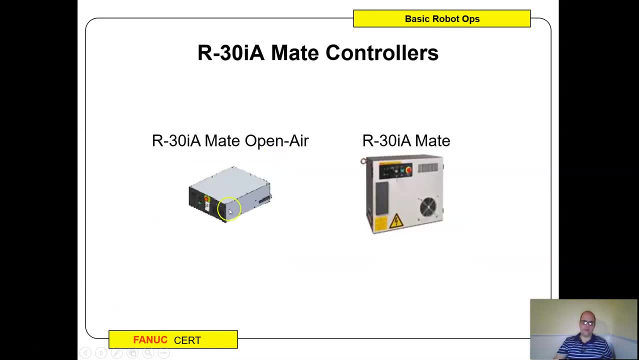 that another, but that's the controller. you know we have an a size controller, b size controllers. for bigger applications we have an a size controller. we have one of these open air mates. this is like if i'm trying to save rack space, i can just put it right in a rack. makes a lot easier. 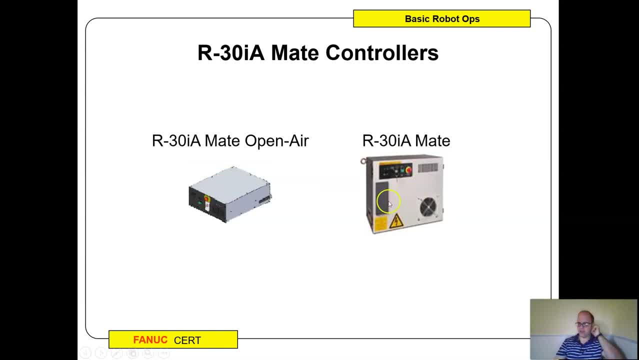 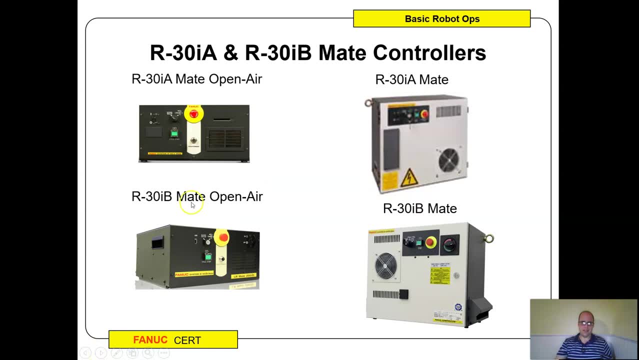 harder to work on, though, trust me. and this is the, the mate controller. it's a lot smaller. this is more like what we have: the r30i a mate. actually, this is our open air right here, now that i'm looking at it again- um, actually, no, it's this one, it's one of them, i think it's this one, and there's the b we have. 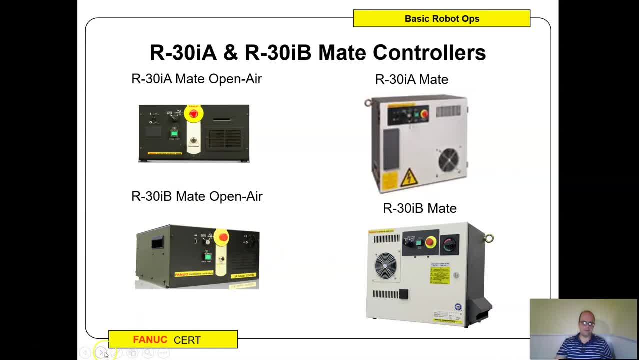 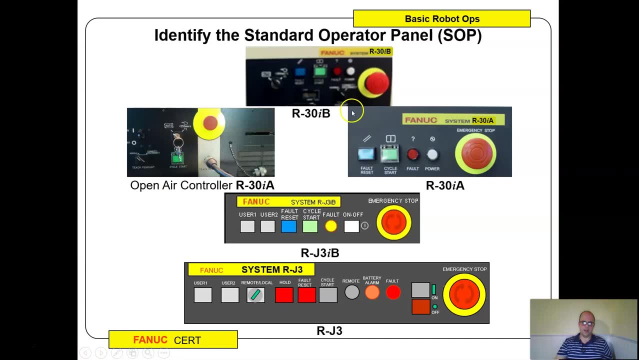 b's at our, our facility. i'm pretty sure i'm almost positive for their bees. and this is: and, uh, there's an operating panel on the controller. um, on the b, uh, you know, yeah, we have a b. there's usually a fault reset, you know. so if i look here there's. 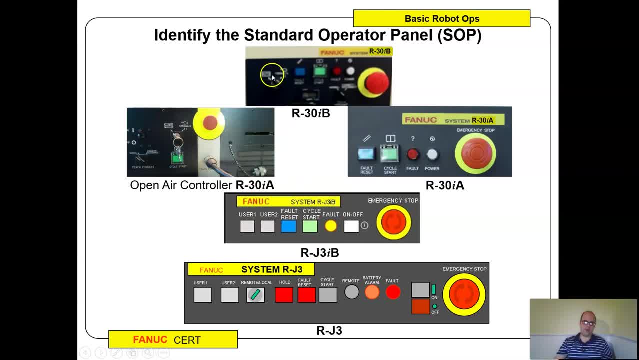 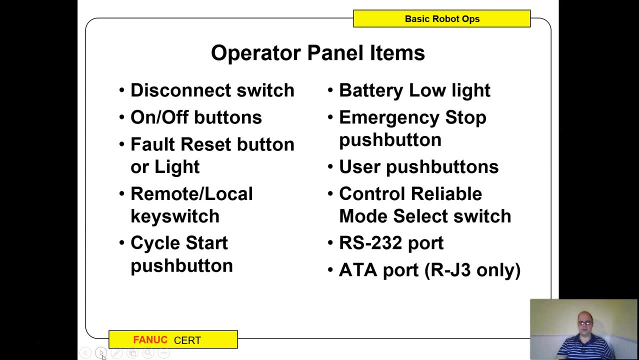 nothing. we don't have these here, but there's usually a, a key that will sets between teach and run, um fault reset, a go button and it tells you if there's a fault or not. and that's how you turn things on. you know operator panels. this is where everything is, at the operator panel. you know user. 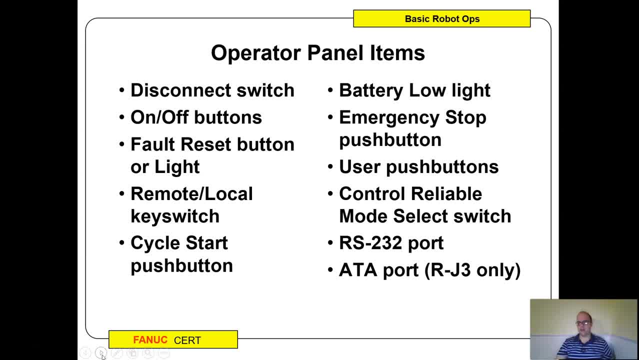 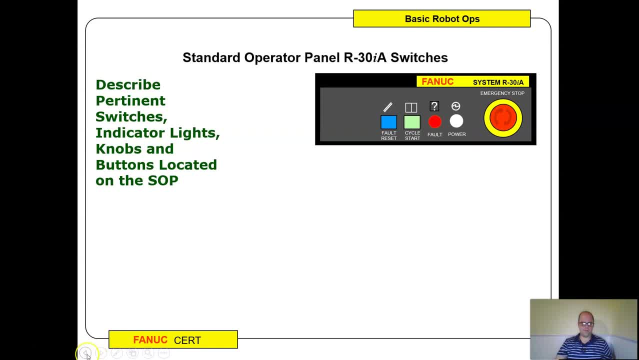 buttons, there's a. you know that's where you start things clear. things can go local, remote, all that fun jazz. um, i'm not going to go through all of this, so, but yeah, emergency, stop the power's on because you want to make sure. and, by the way, red means on, because red means power. 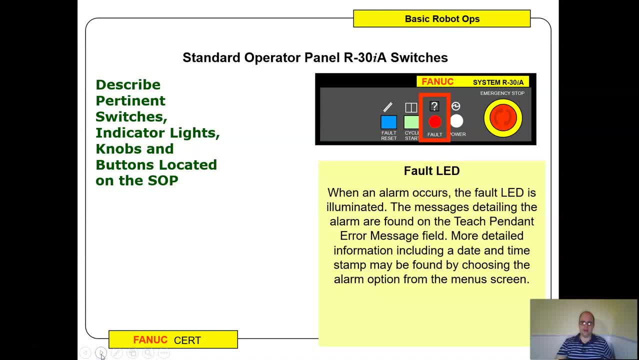 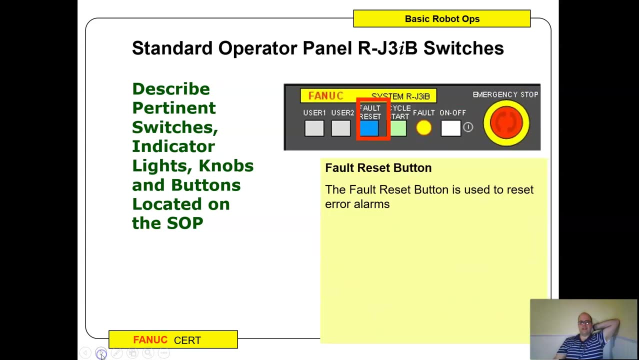 or unsafe to enter and you can see the fault led when it turns up. um fault reset will help reset anything. there's also something on the teach pendant as well, but then cycle start is the you know green button that starts things when you're in automatic, and i'm just going to advance through this. these user buttons could be something you set up, if so, 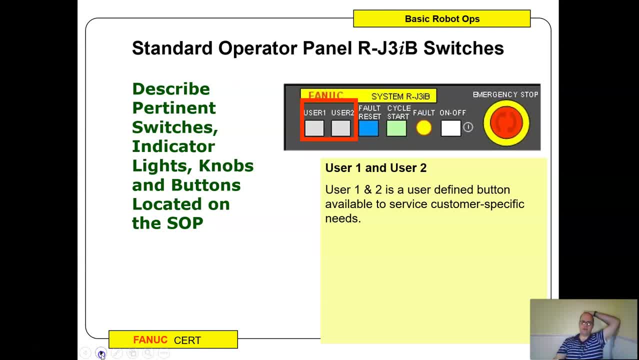 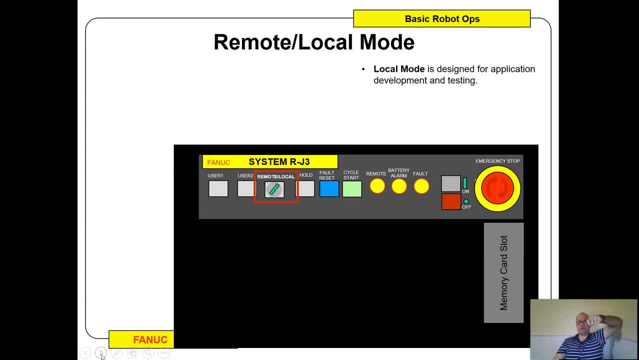 if you wanted to run a macro or something, that's where you could use those buttons on the um. and then one other thing: local, remote. local is for testing. this is what we're usually going to be in. remote will allow us in production to run things off of a plc or another controller or something. 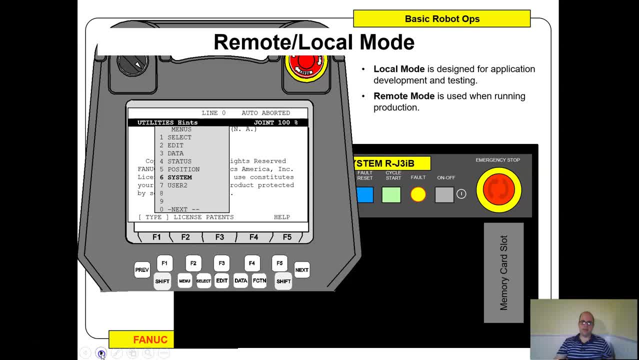 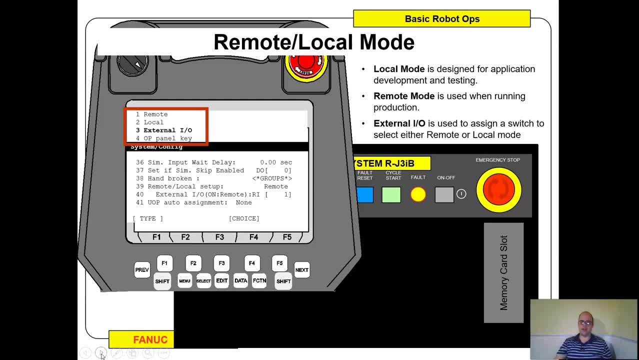 along that line: um, so that's, that's what we're going to do. and then we're going to go ahead and lines: um, so yeah, and this talks about how you set that up. i'm not going to even worry about that right now. you could also in your i o set up to run off and not turn on, i o start. that's a different. 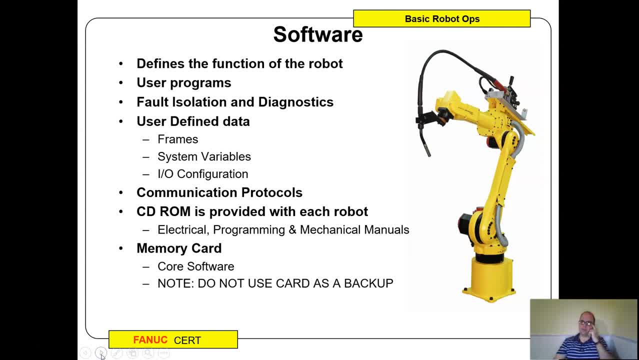 class. again, the software is all there, um, it's pre-loaded. make sure you always back up with images. we'll talk about another, another, because if things go down you're in trouble and you got, and it pays a lot of money. so this, there is software and it would always back up with an image. 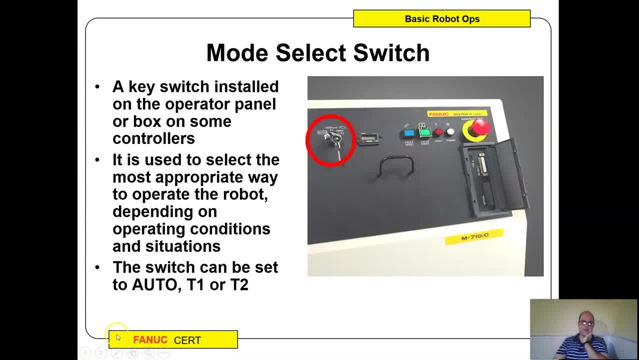 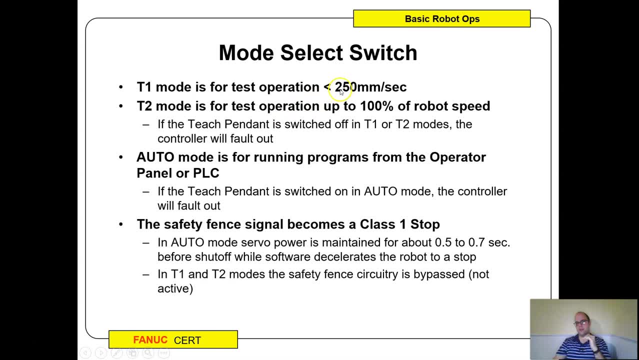 mode select. there are three modes that you can run things in. t1 mode is is going to limit you to, uh, only 250 millimeters per second. t2 is a test operation mode. um, but it it will. um, let you run up to 100 speed, but it's still in teach mode, meaning it won't. 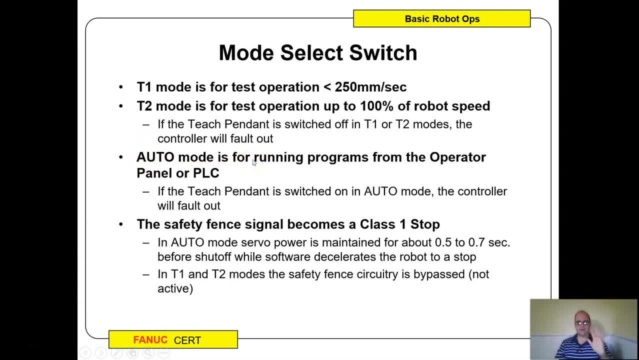 you have to control it with a teach pendant. auto mode that's straight out the gate. go for it. um, uh. and now keep in mind: if safety fence is a class one, stop so when it goes in auto mode. if you're, if it's safety fence violates, servo power will be maintained for a second or two, but then it'll. 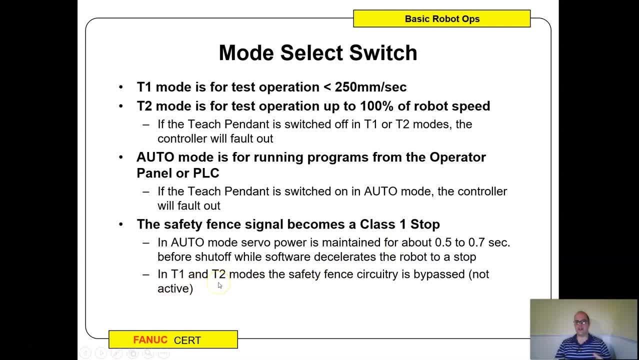 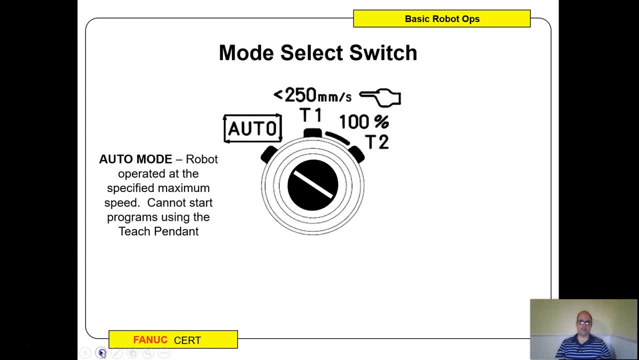 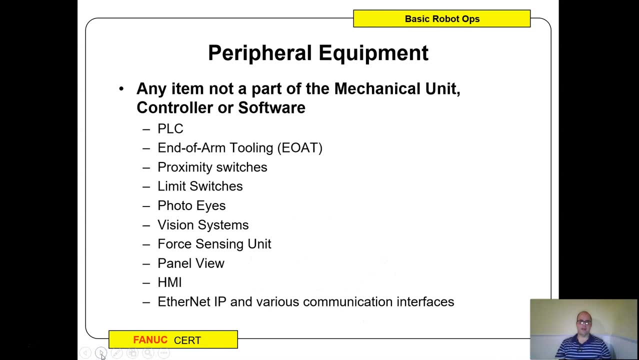 stop and break the robot um t1. t2 will allow safety fence stuff to be bypassed because you might be in there doing stuff. so just keep that in mind. here's what it looks like and you can see see here. uh, peripheral equipment- plc- end of arm. 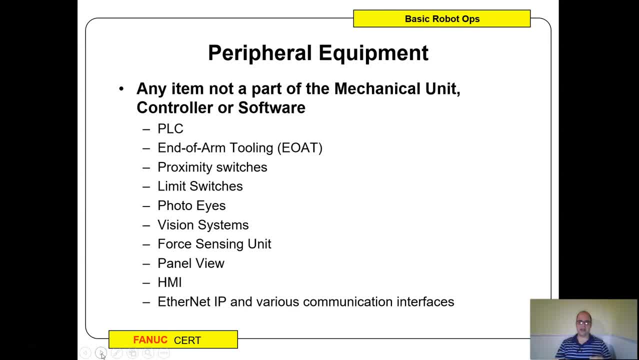 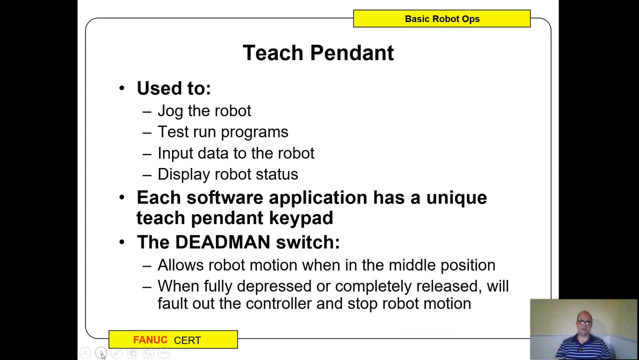 tooling, hmi. we have some hmis directly tied into our robots for an i o, simulator cameras, vision systems. we have those as well, you know. so this is some of the stuff, like teach pendant- we talked about the dead man earlier. it's got to be in the middle position, but this is where 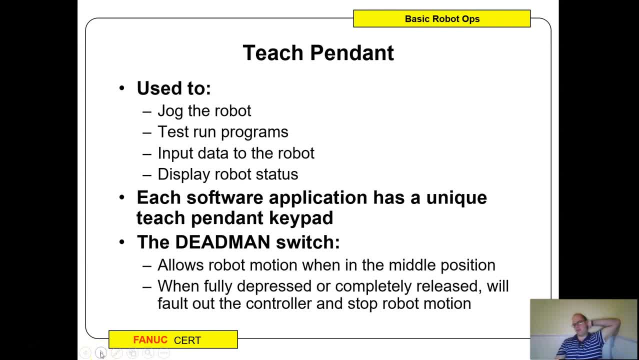 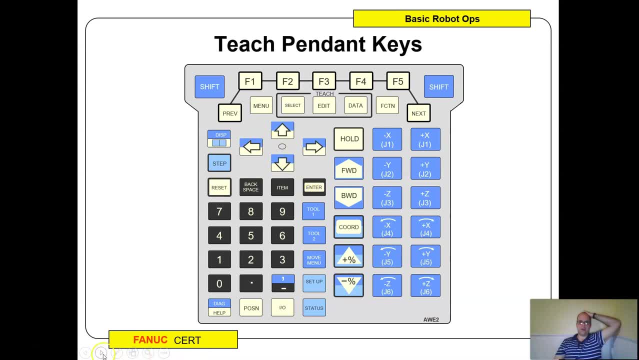 we do all of our programming. um each, every, every button has unique application. we'll talk about that in future classes. um, here's some of the the pendant pendant keys. this is what it basically looks like. you know, when in doubt, always hit the previous button. um shift is anything that's in blue. you need to hit shift in order to execute it. so 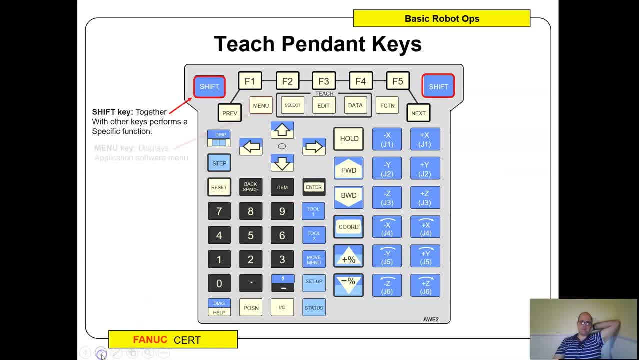 just keep that in mind. oftentimes, and in in uh, session one, there's a whole breakdown. all this menu is where you're gonna get a lot of your stuff. you know where you're gonna find a lot of your like settings and configurations. uh, these work as cursors up and down if you hold 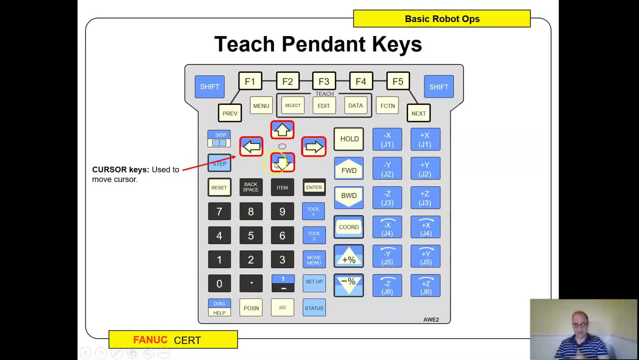 down shift. think of it in one of these buttons. they'll be like: skip down fast um step mode. this is key. you'll hit this button if you wanted to go. go all the way through your job, or one step at a time. i always recommend, when you're first testing out, step it through. 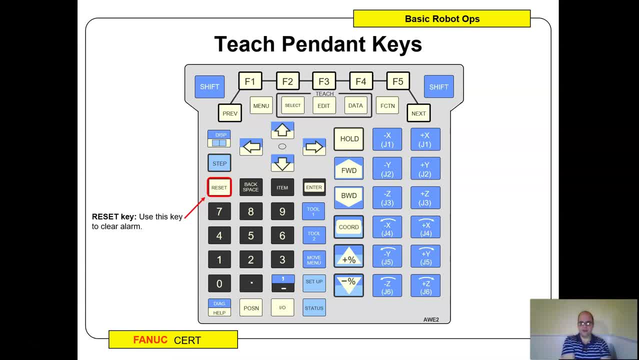 reset. that's gonna be your friend that clears your alarm. so when in doubt, hit reset i would. i would know the three buttons i would know previous: reset. enter- those are the ones you use a lot. um, some of these we'll talk about in the classroom, but enter. 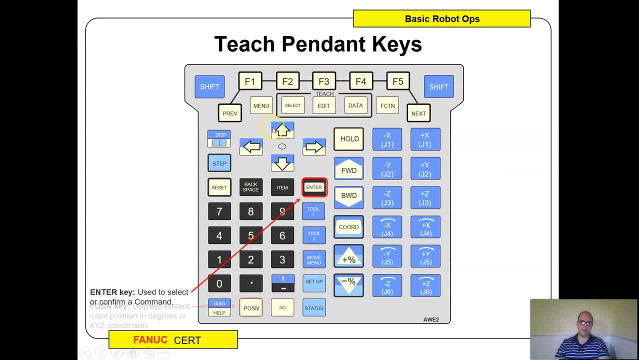 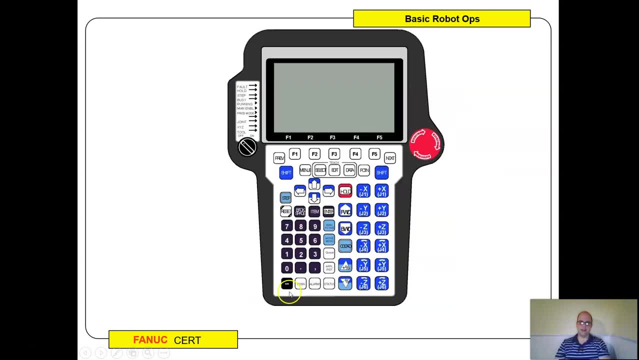 you know pre previous reset, enter next these salt. i would. i would know three buttons. i would know previous reset, enter next these salt soft key buttons. position: io: again some of the stuff we'll hit in other classes so i'm not going to talk about too much. this will tell you your current position in the site. 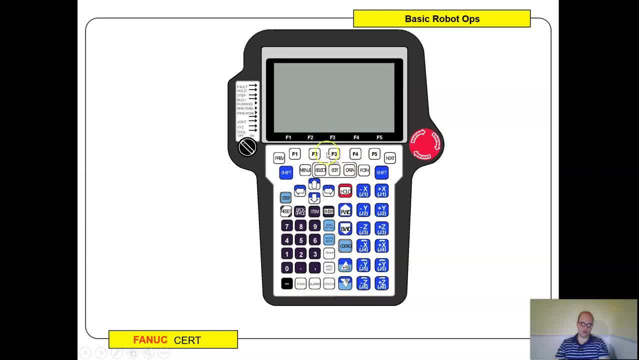 condition to io. this is what the old controller looks like, because it has display indicators right here and turns things on and off. we have a controller like this and some robots run this this way. our newer controllers- all the status lights are up at the top here because 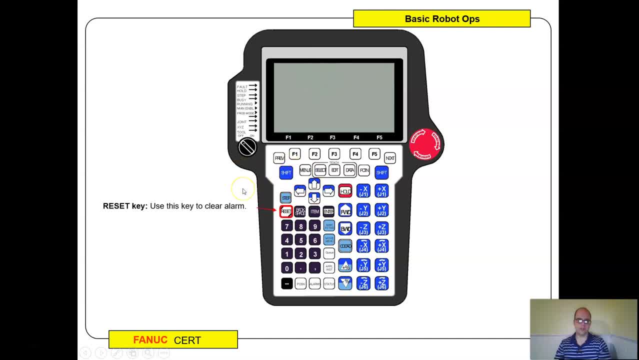 it's led, so it's just fyi. same buttons, just maybe in a different area. so i'm just going to advance through. it's all in the powerpoint. forward, you know, forward buttons and backward buttons allow us to like run the job through through the commands, but when we get to class, you're going to hold down. basically you're going. 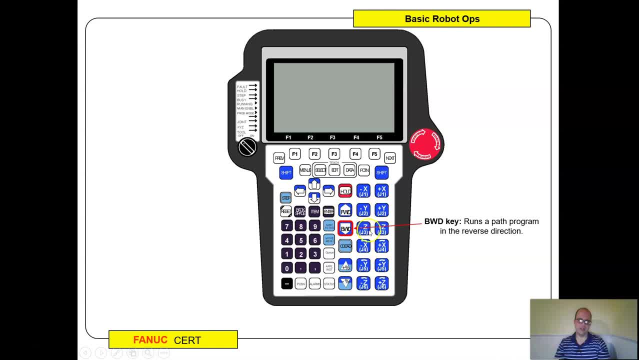 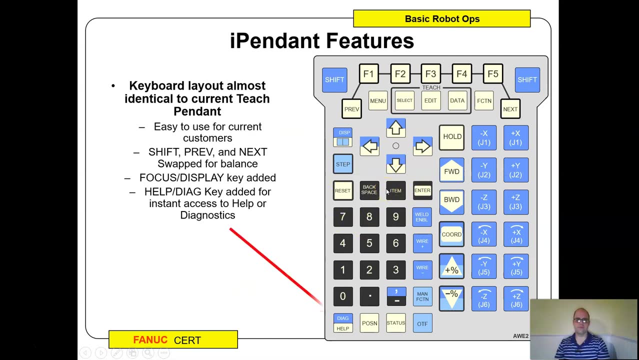 to turn on the robot: hit, reset, hold down, shift and use these buttons to jog. simple as that. there's a teach pendant, there's the led screen and the function keys. you know, some of this is straightforward. this is the pendant that we have. yeah, this is more like it. all the status lights. 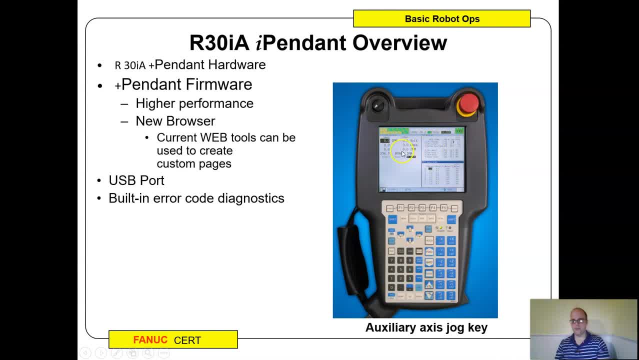 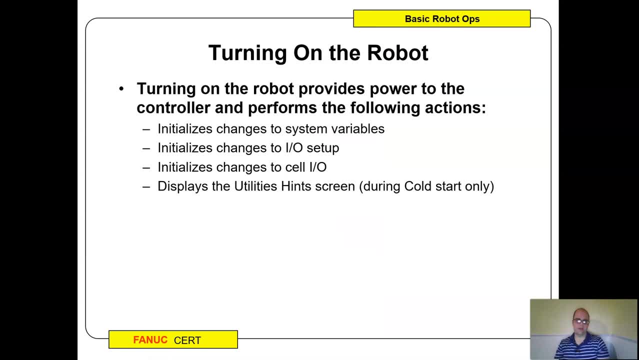 are appearing up here. this is all touchscreen and you can, in theory, put in a mouse and a keyboard too, so just keep that all in mind. turning on the robot, you flip a switch in our classroom. you know you want. you're probably not powering out too much, but that's you know. you always want. 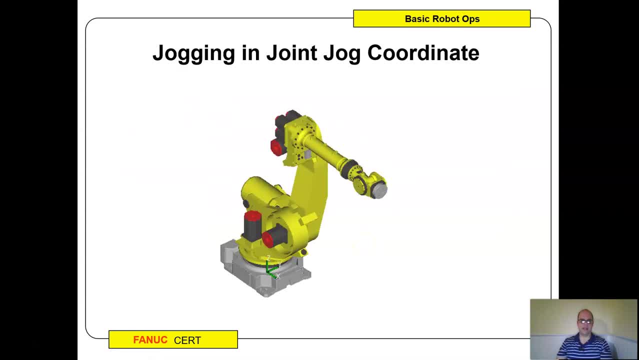 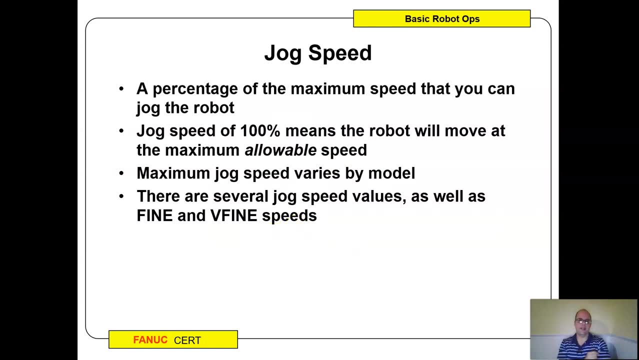 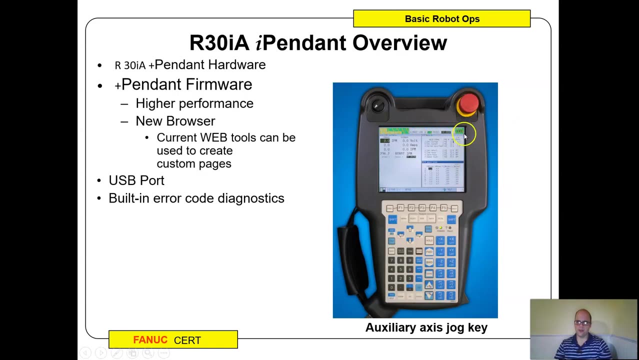